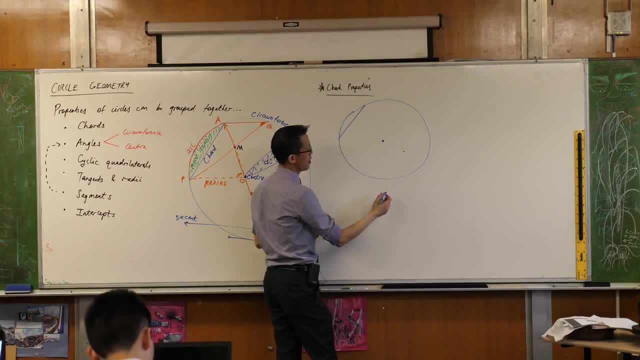 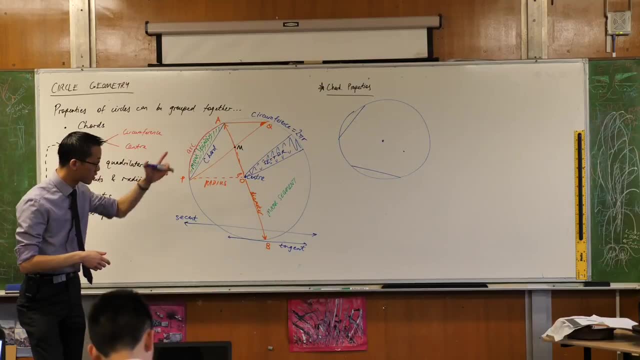 Maybe something like: over here and over here. okay, You can make them short, you can make them long, you can make them overlap, you can make them not touch each other- like mine don't, Once you've made them the same length. 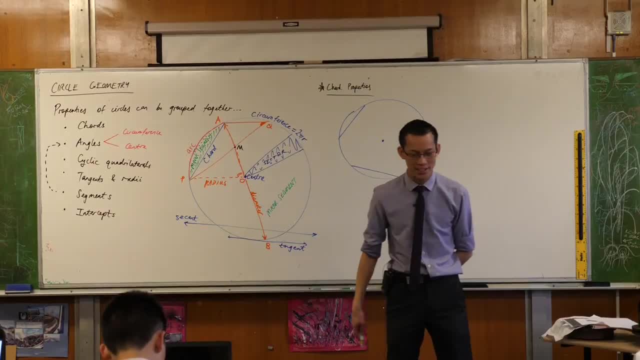 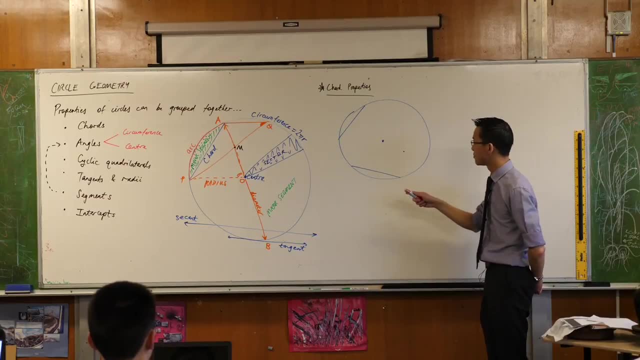 and it'd be really nice, by the way, if you had these different to the person next to you. I then want you to join from your cord the shortest distance from your cord to the center. I'm not going to draw it in just yet. I want to give you a moment to try this out yourself. 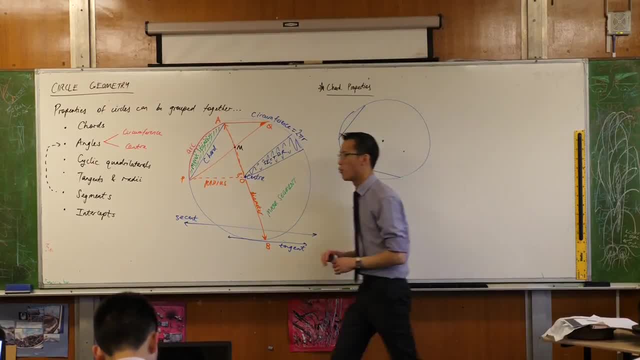 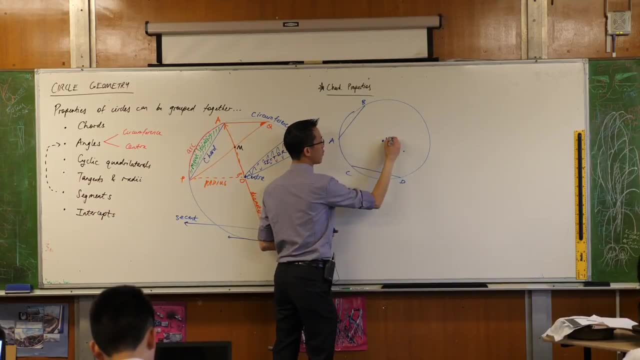 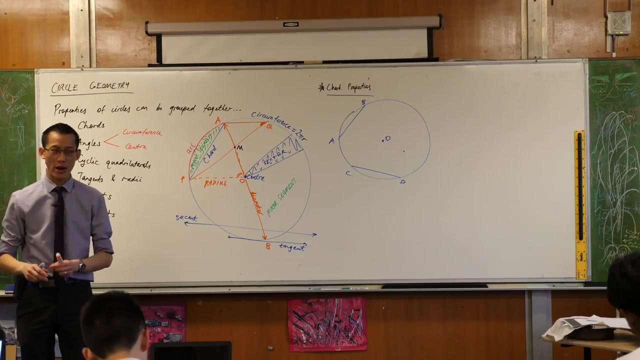 You've got two chords here and we'll give them some names, shall we? Let's call this one AB, let's call this one CD. you've got your centre O. I want you to join AB and CD to the centre in the shortest way possible. 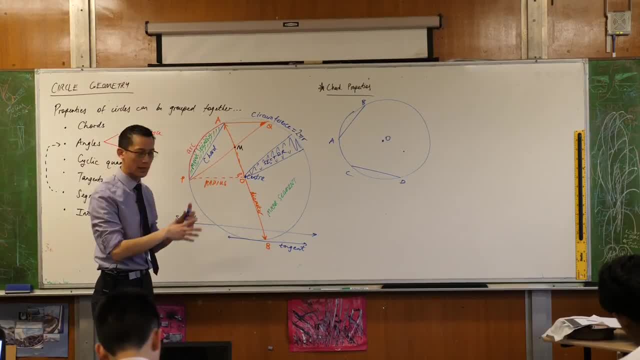 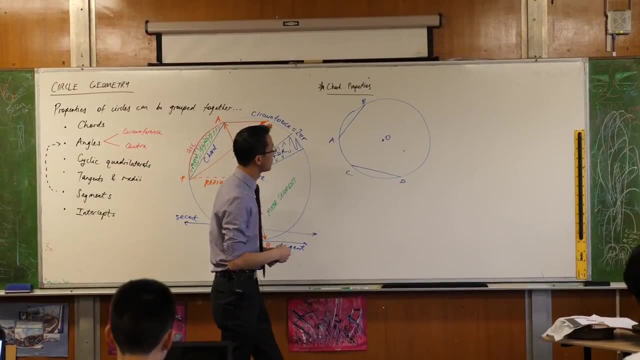 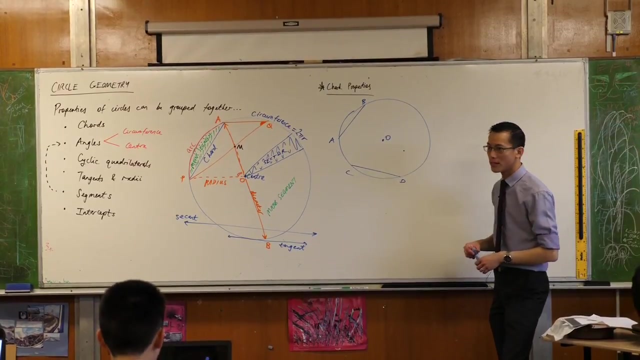 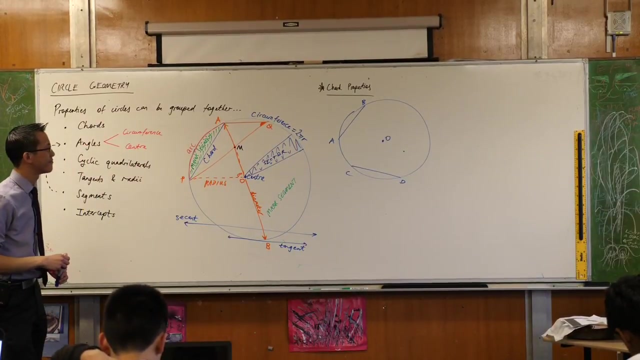 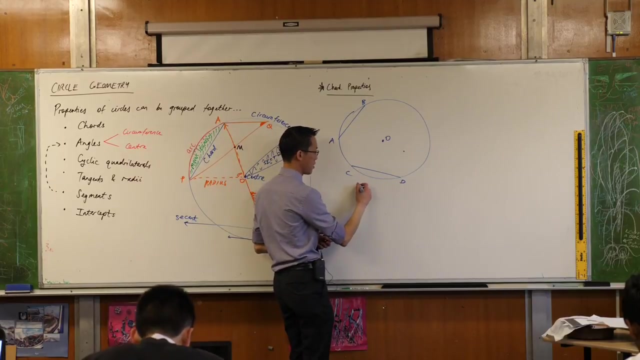 Can you do that? I'll give you a second to catch up. Make sure you've got everything labelled out. You, alright, Jake. So you've got two chords. they're the same length, So maybe underneath this you want to write: chords AB and CD are equal. 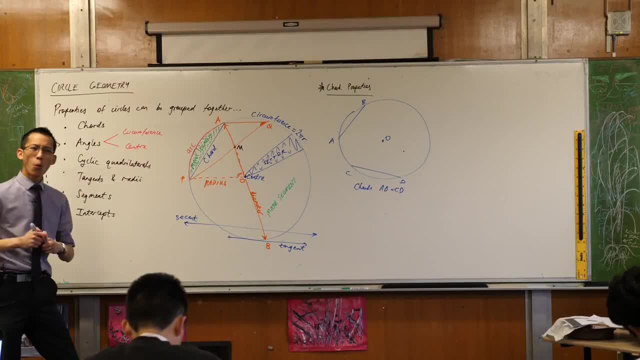 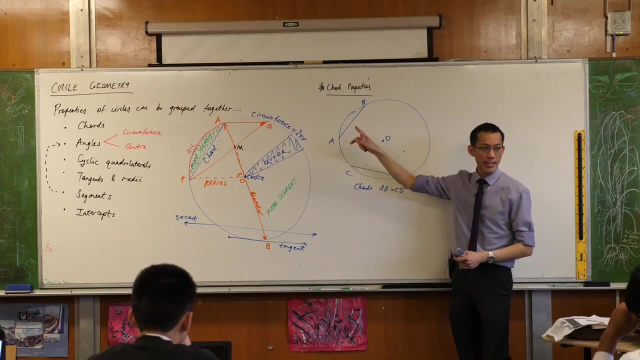 We'll label them. We'll label them as equal in a second When you join up your chords to your centre. I said the shortest length. The shortest length between a point and a line is not just any length, it's the perpendicular. 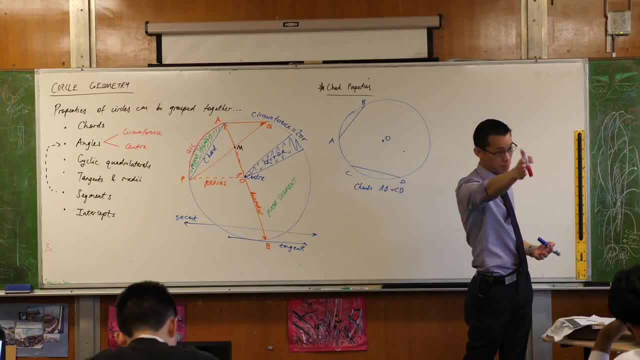 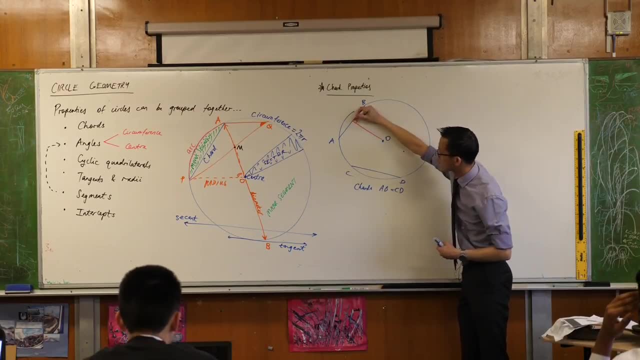 That's the quickest way across, just like crossing a road, The quickest way across the road is straight across the road. don't take it at an angle. So if you join these up and you mark in the right angle, which indicates that's the shortest distance, you can get. 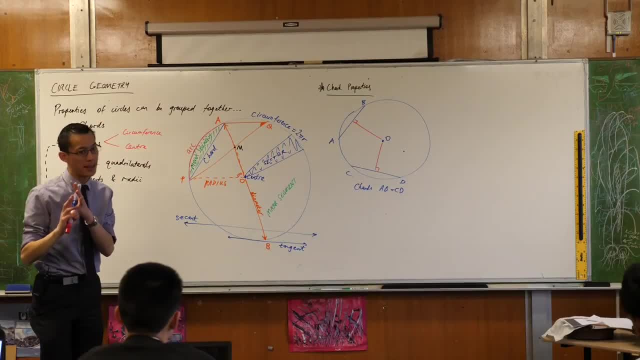 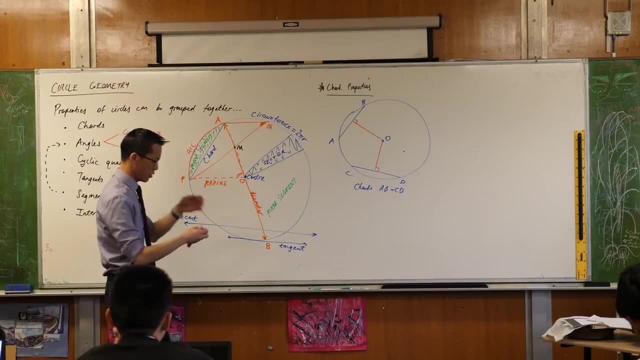 Remembering that I didn't give you any instructions about how long to make your chords. I just said: make them the same. I didn't tell you where to put the chords. I said: put them anywhere you like. I want you to have a look at these two lengths that you've just drawn. 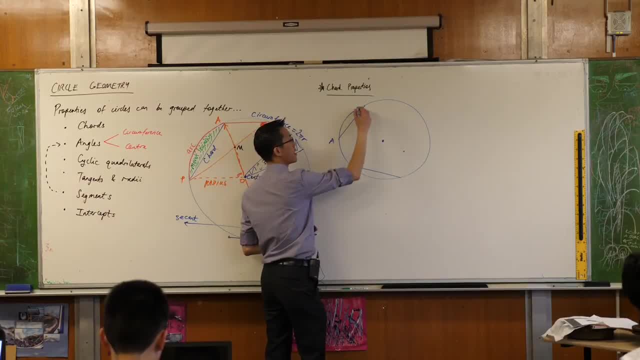 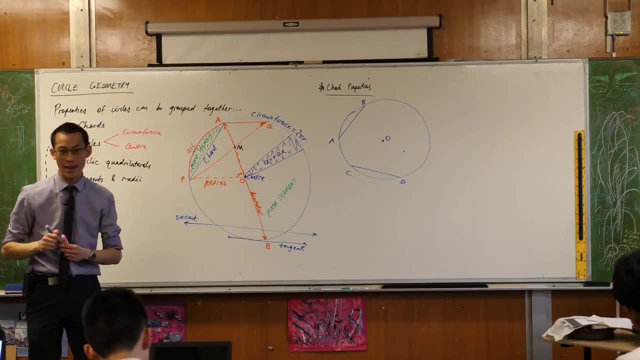 some names, shall we? Let's call this one AB. Let's call this one CD. You've got your center O. I want you to join AB and CD to the center in the shortest way possible. Can you do that? I'll give you a second to catch up, Make. 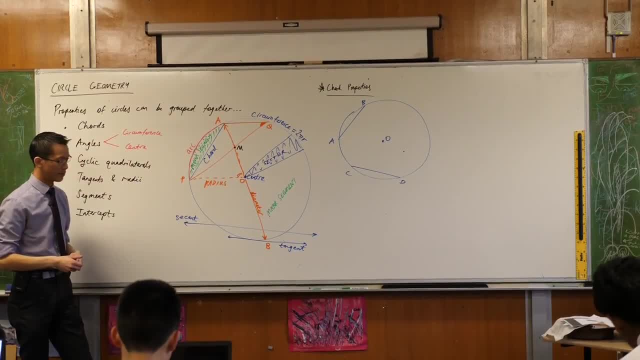 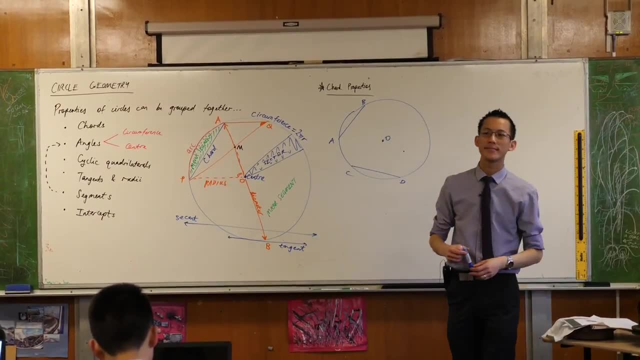 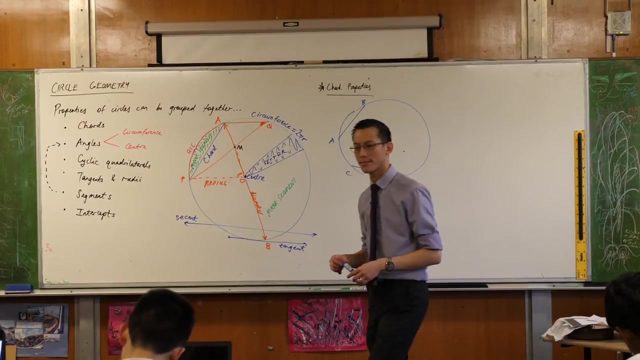 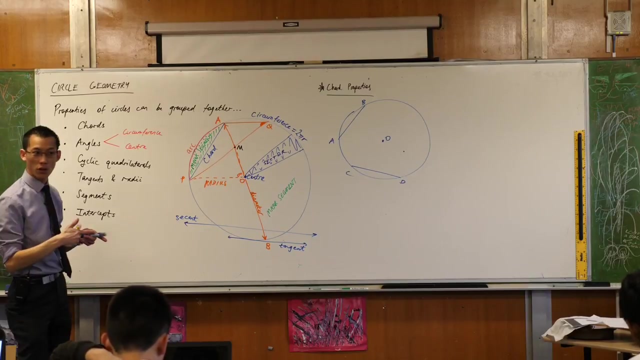 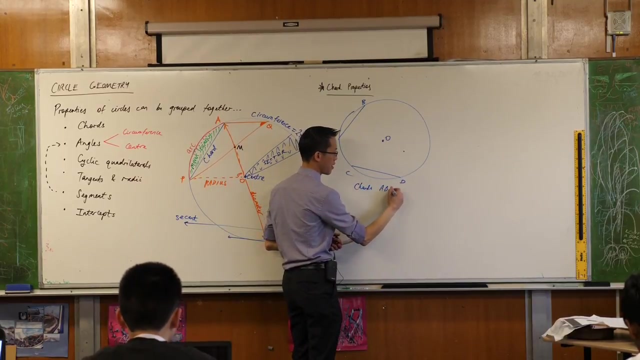 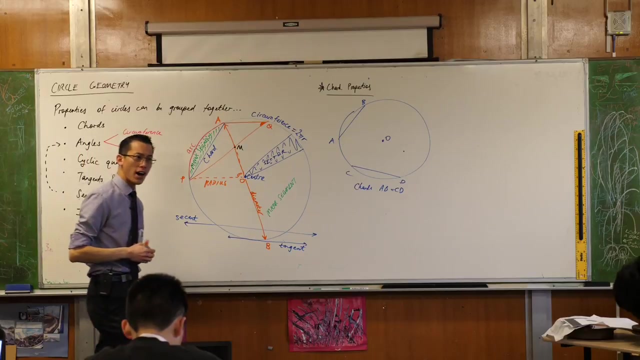 sure you've got everything labeled out. You're right, Jake. So you've got two cords. They're the same length, So maybe underneath this you maybe want to write: cords AB and CD are equal. So you've got to write the cords AB and CD are equal. OK, We'll label them as equal in a second. 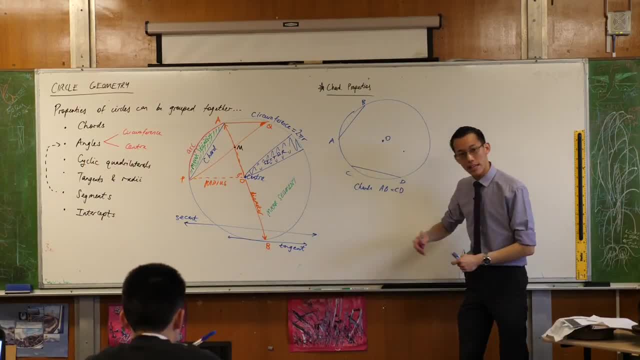 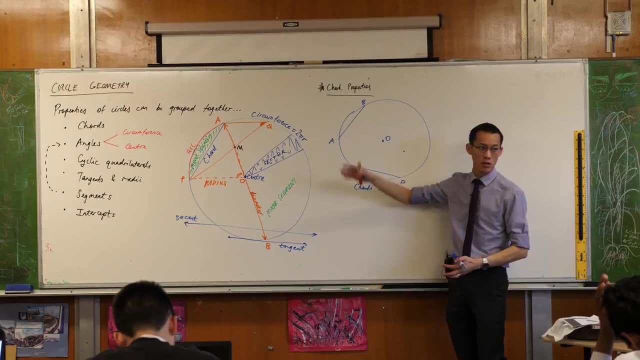 When you join up your cords to your center. I said the shortest length. The shortest length between a point and a line is not just any length, It's the perpendicular right. That's the quickest way across, Just like crossing a road. the 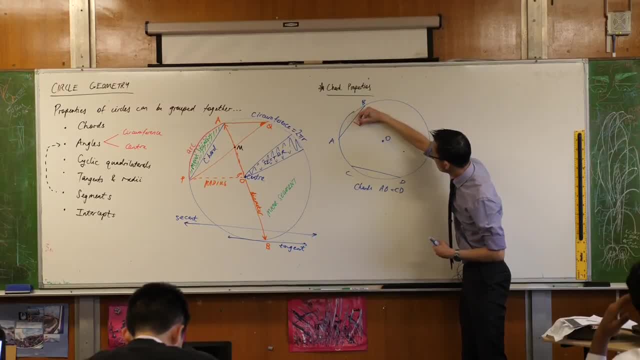 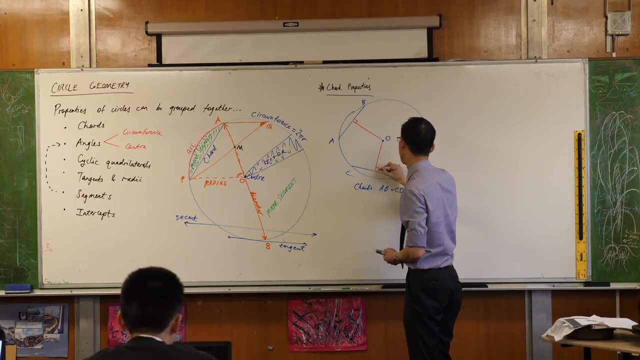 quickest way to cross the road is straight across the road, Don't take it at an angle. OK, So if you join these up and you mark in the right angle, which indicates that's the shortest distance you can get, Remembering that I didn't give you any instructions about how long to make your chords. I just said make them the same. 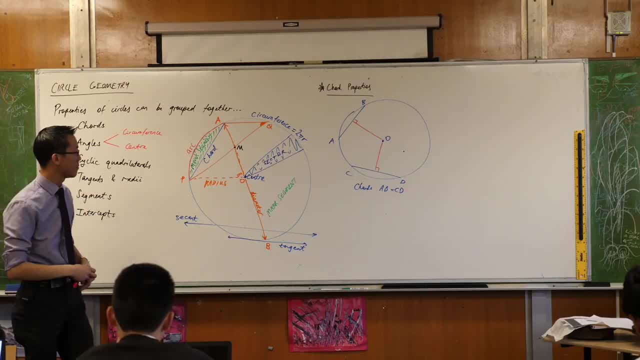 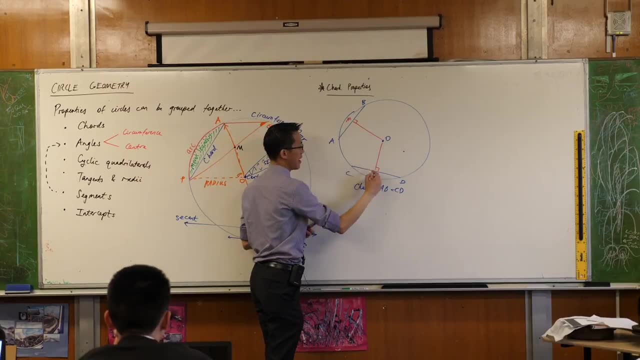 I didn't tell you where to put the chords. I said: put them anywhere you like. I want you to have a look at these two lengths that you've just drawn. Let's call them OM and ON. When you look at it, you can almost see. 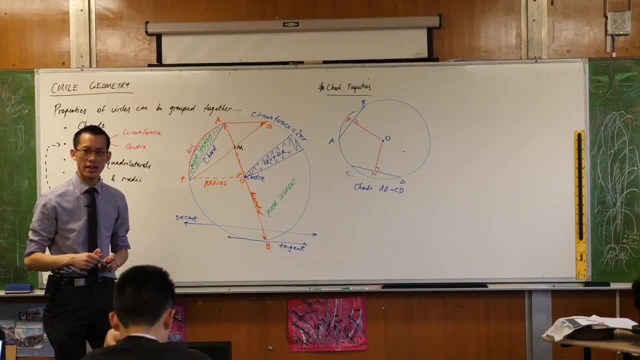 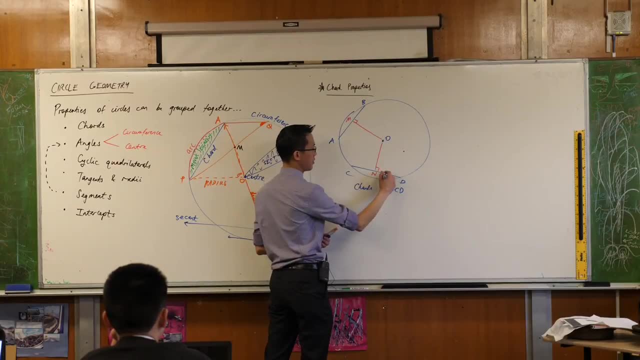 And when you measure it, you should be able to confirm. what do you notice about these two lengths? They should be equal. they should be equal. So I'm now going to mark in that CD and AB are the same And, along with that, OM and OM are the same. 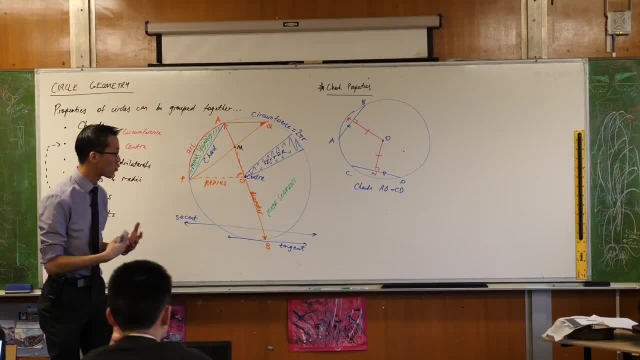 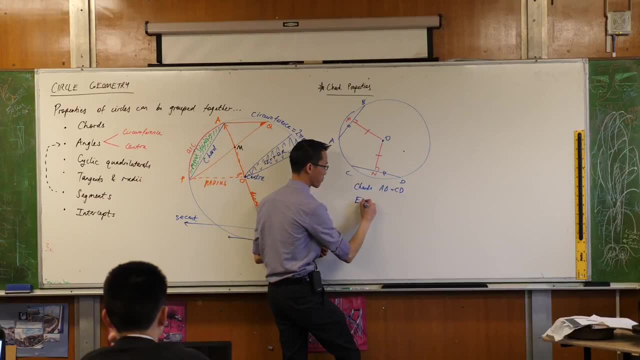 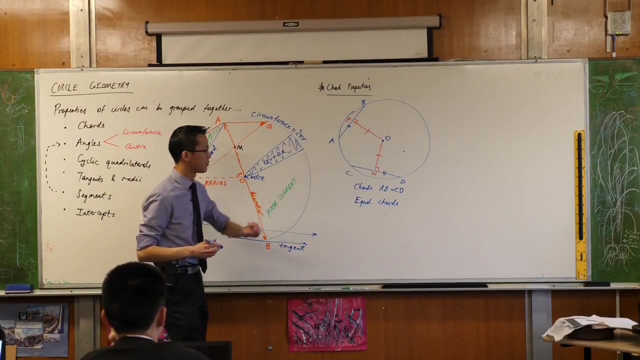 Okay, so how could we word this? What's a way that we can describe what's going on? We started by saying: equal chords. What are they? What do they share in common? How would you describe the fact in words, verbally, that these two distances are the same? 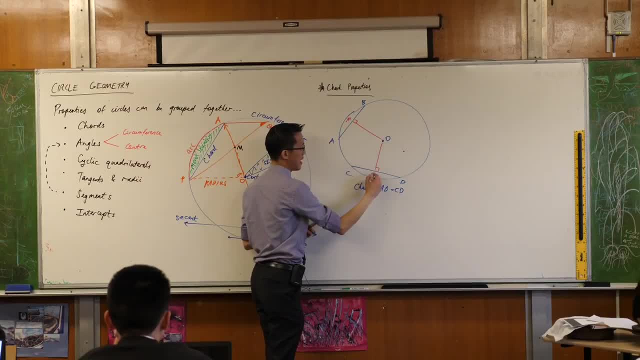 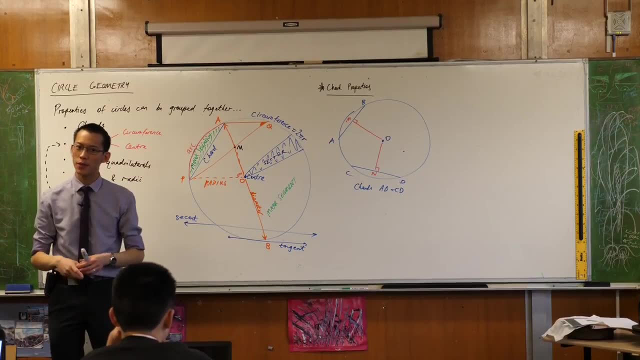 Let's call them OM and ON. When you look at it, you can almost see, And when you measure it, you should be able to confirm. what do you notice about these two lengths? They should be equal. They should be equal. 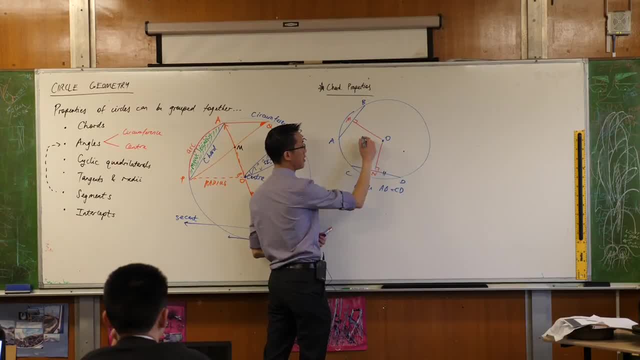 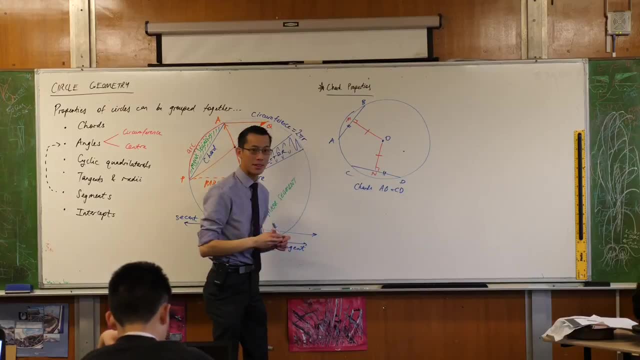 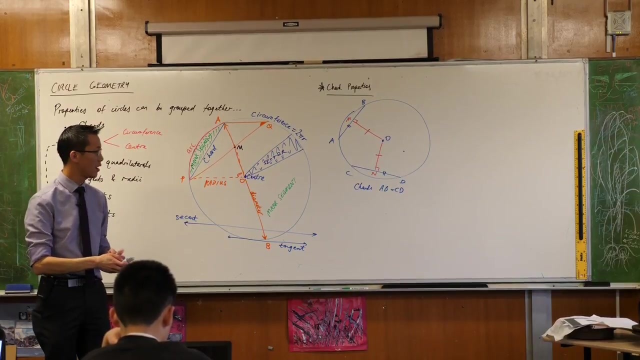 So I'm now going to mark in that, once you mark in that CD and AB are the same And, along with that, OM and OM are the same, Okay, so how could we word this? What's a way that we can describe what's going on? 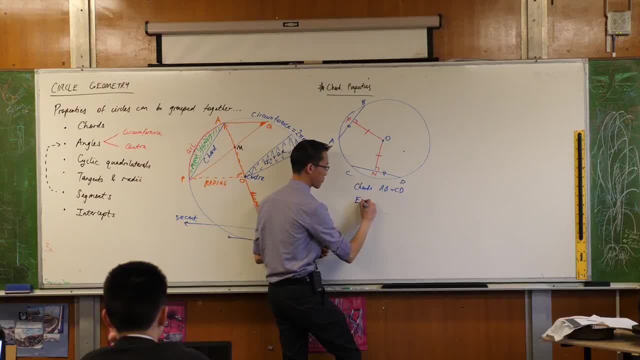 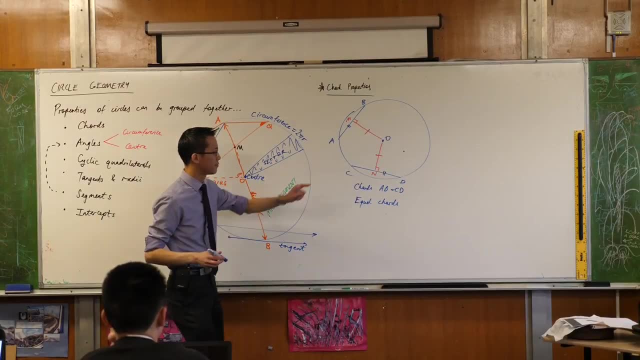 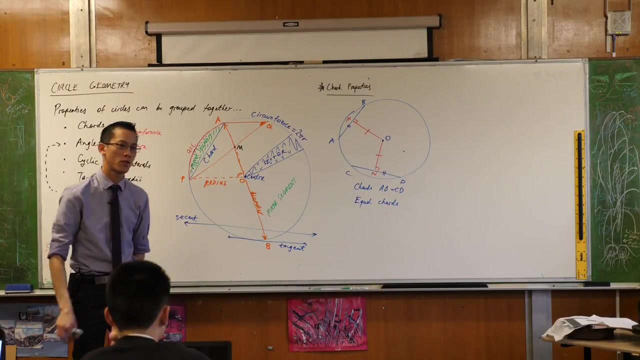 We started by saying: equal chords. Equal chords. What are they? What do they share in common? How would you describe the fact in words, verbally, that these two distances are the same? We want to make this as succinct as possible. Use as few words as you can. 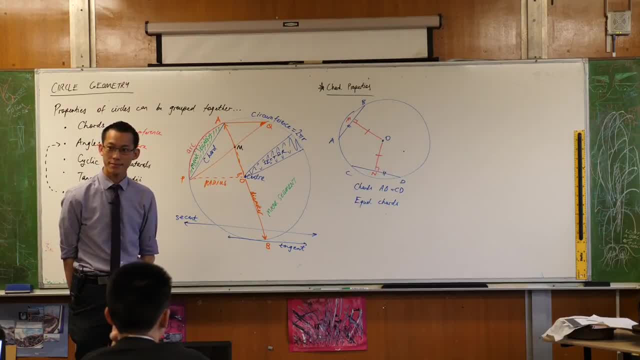 Say that again. If they're equal, then what's left of the radius? What's left of the radius? Okay, just watch out. We've got all these features here. I want to point out I haven't drawn any radii on this circle. 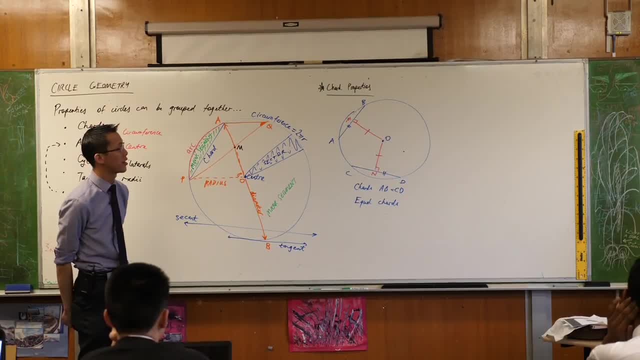 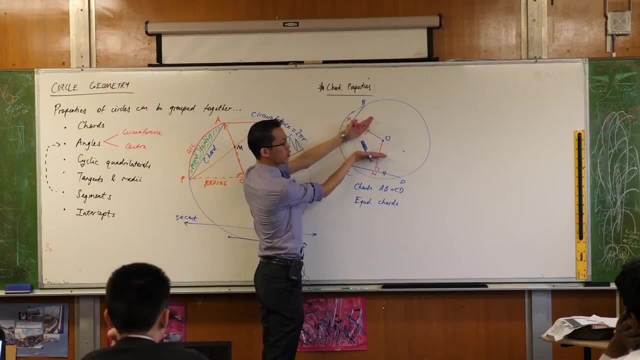 There are no radii that have been constructed because I've never joined the centre to the circumference. I've gotten close, but I haven't. I could make it even more obvious that I haven't by putting these chords closer to the centre. 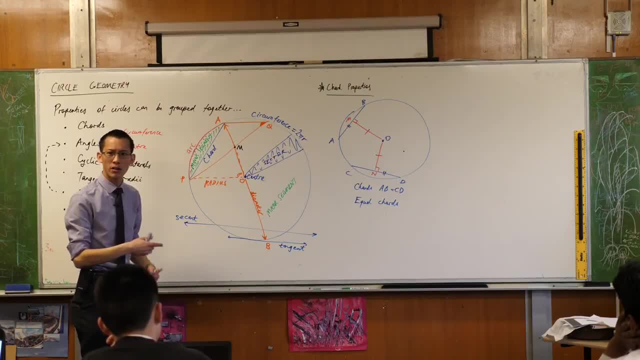 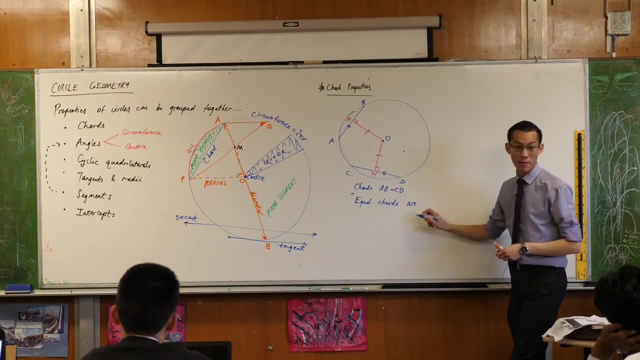 It's obviously not a radius. So how would you describe what's going on here? Equal chords are So again, remember, we're trying to use as few words as possible. I'd probably say that being that they're the same distance from the centre. 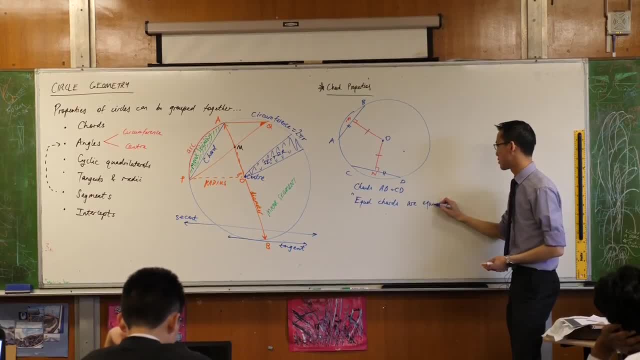 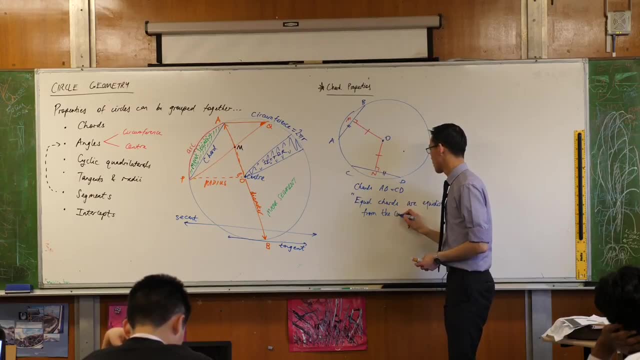 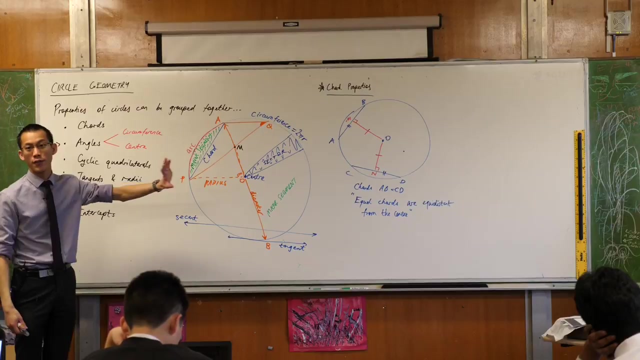 the word I would use is equidistant. Okay, Now I apologise. We're sort of doing this a little bit in slow motion, because this is the very first chord property that I'm mentioning. You guys are going to do this on your own for some of the later ones. 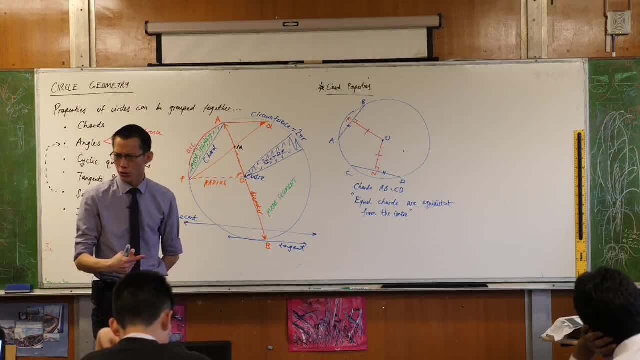 How are we going to prove that this is the case? Like it looks true. You've measured it well within the limits of your measuring instrument. It looks pretty true, But how can you prove it? You remember we had a look at the parallel lines and transversals last time. 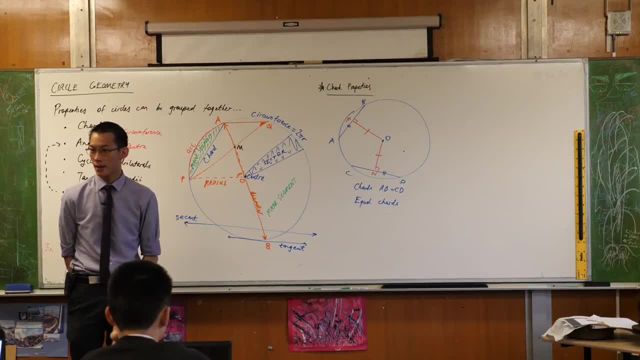 We want to make this as succinct as possible. Use as few words as you can. Say that again: If they're equal, then what's left of the radius? Okay, just watch out, We've got all these features here. I want to point out I haven't drawn any radii on this circle. 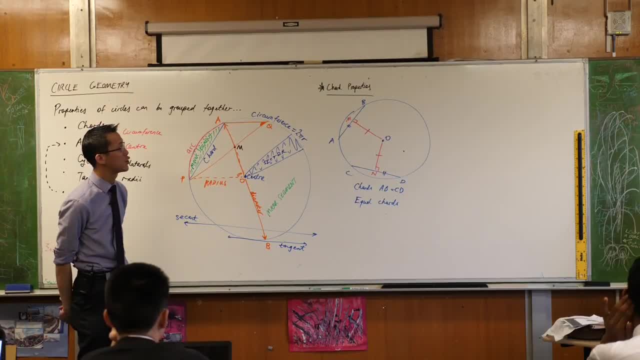 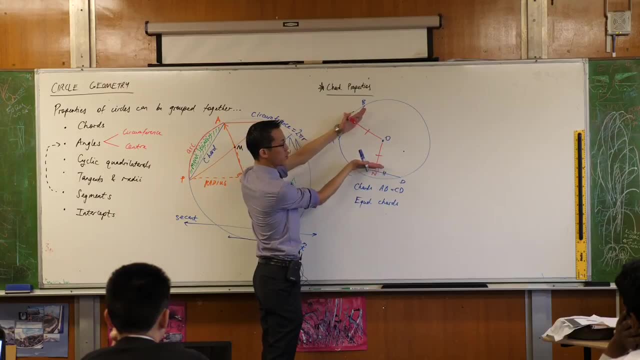 There are no radii that have been constructed because I've never joined the centre to the circumference. I've gotten close, but I haven't. I could make it even more obvious that I haven't by putting these chords closer to the centre. 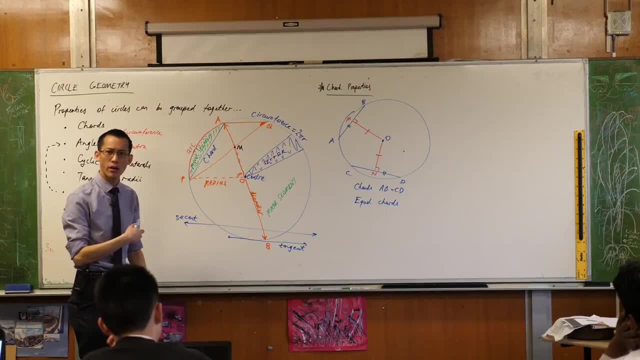 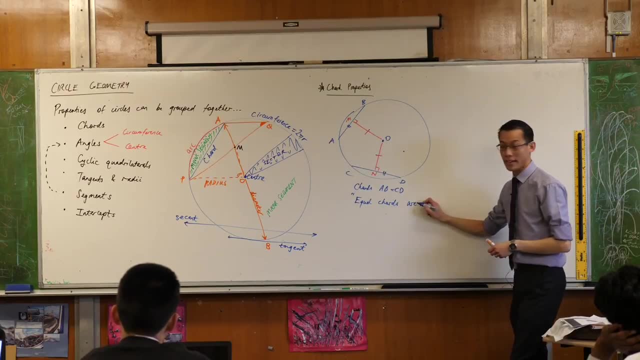 It's obviously not a radius. So how would you describe what's going on here? Equal chords are So again, remember, we're trying to use as few words as possible. I'd probably say that being that they're the same distance from the centre. 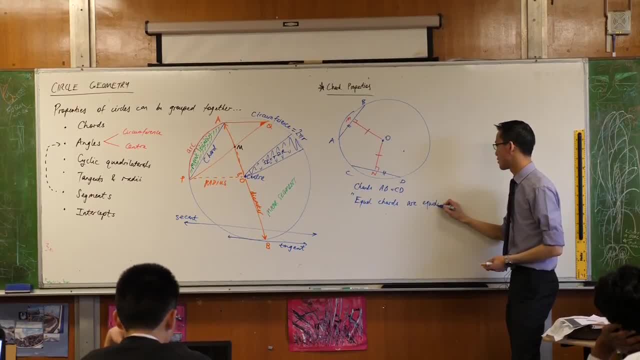 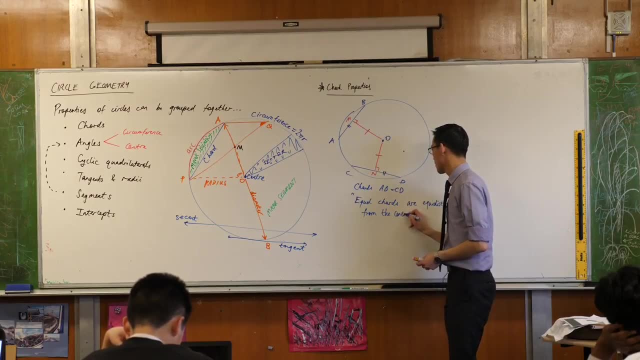 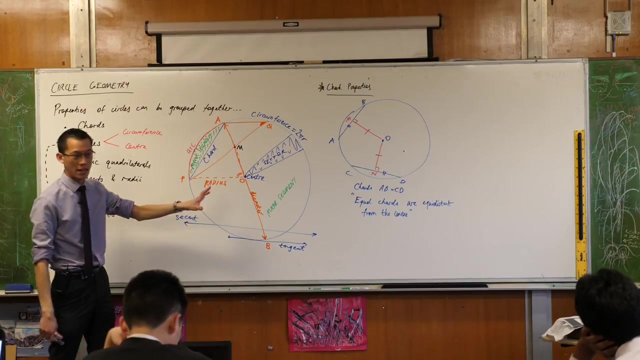 the word I would use is equidistant. Okay, Now I apologise. we're sort of doing this a little bit in slow motion, because this is the very first chord property that I'm mentioning. You guys are going to do this on your own for some of the later ones. 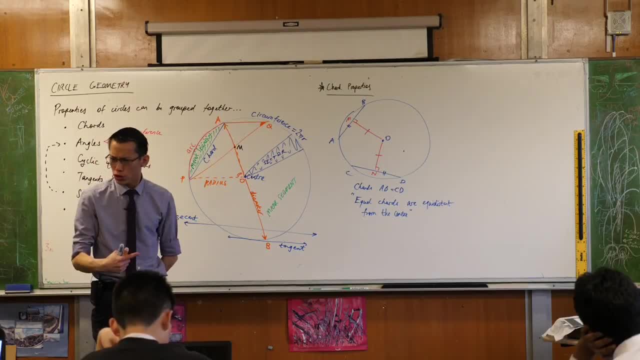 How are we going to prove that this is the case? Like it looks true. You've measured it well within the limits of your measuring instrument. It looks pretty true, But how can you prove it? You remember we had a look at the parallel lines and transversals last time. 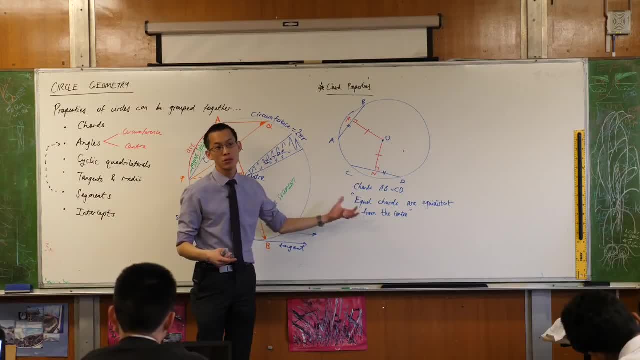 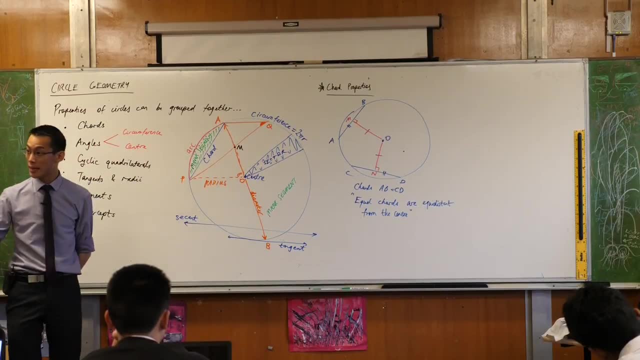 We said it looks good, Measured it, We all tried it, but we proved it using logic. How would you prove that this is actually the case? Anyone want to make any suggestions? Say it again. Okay, we could launch with Pythagoras. 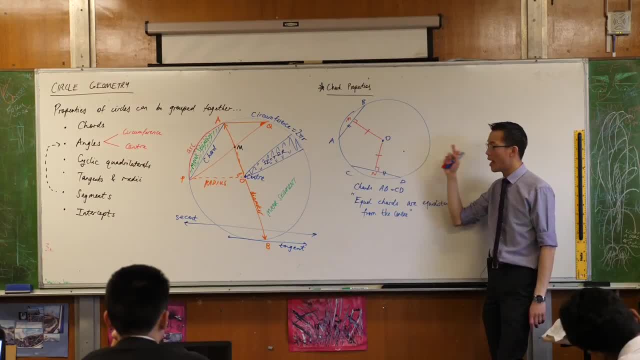 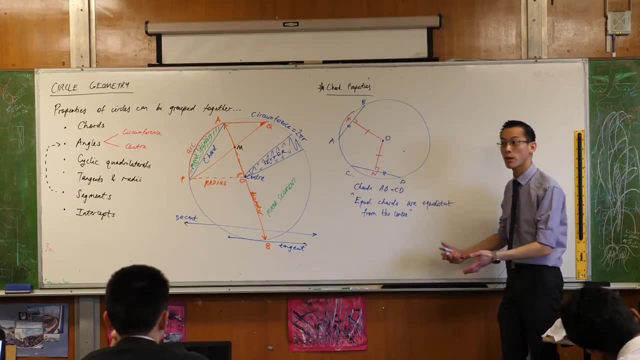 Pythagoras is a sort of logical way to go because you see right angles. However, it's also illogical because I see no triangles. So would you like me to put some triangles on here? Yeah, What triangles would you like me to draw? 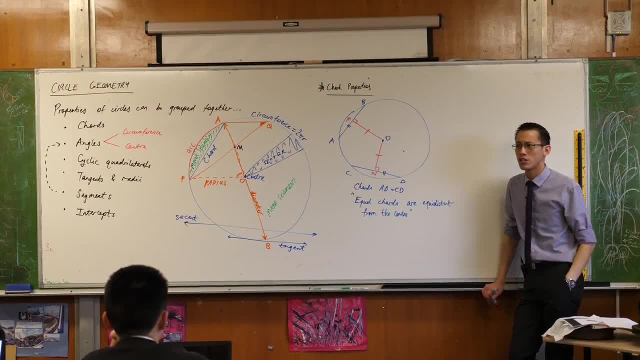 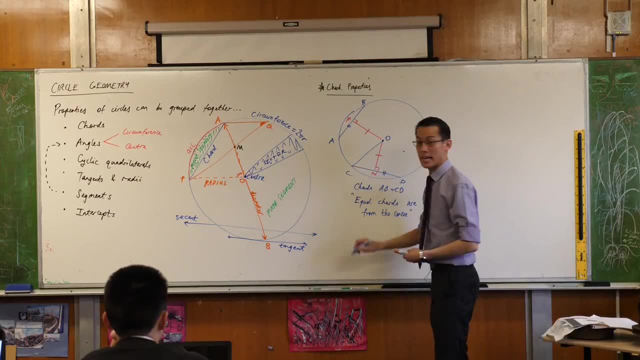 Tell me You've got words, you've got labels. Tell me what I need to join up: C and O, C and O, Like that. Is that enough? Do I need to join up anything else? A and O, A and O. 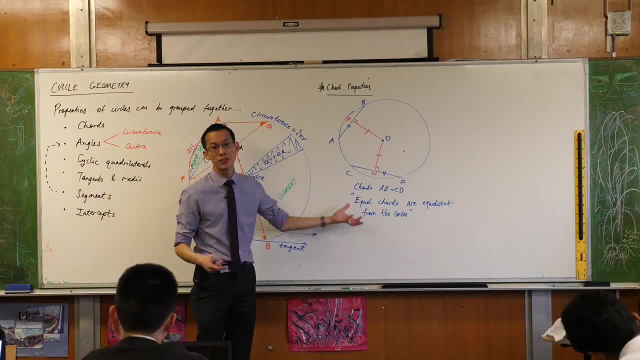 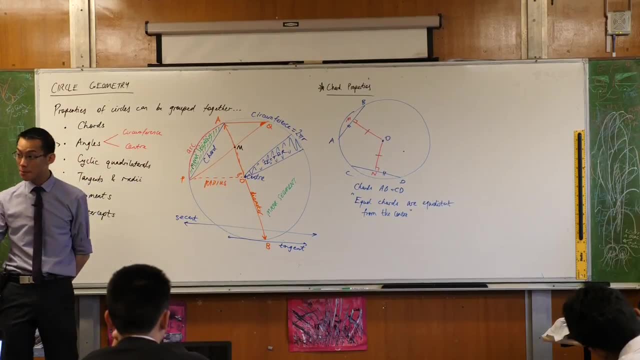 We said it looks good, Measured it, We tried it, But we proved it using logic. How would you prove that this is actually the case? Anyone want to make any suggestions? Say it again. Pythagoras- Okay, we could launch with Pythagoras. 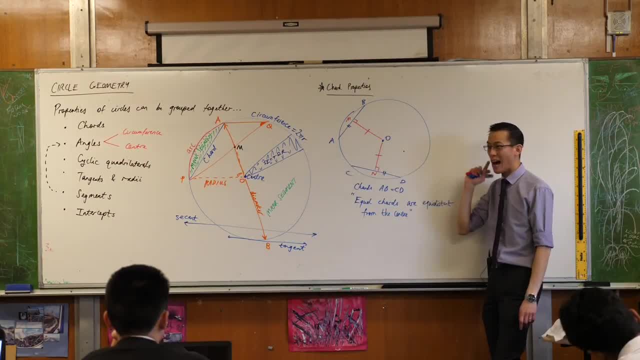 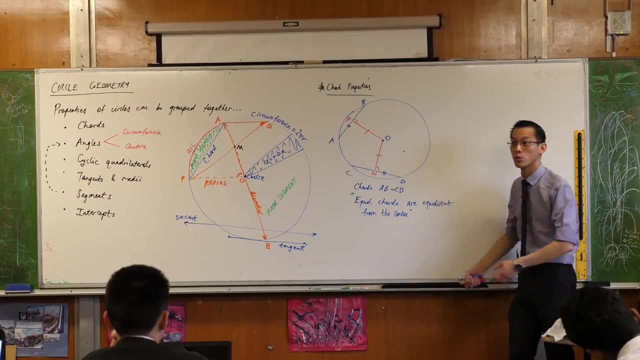 Pythagoras is a sort of logical way to go because you see right angles. However, it's also illogical because I see no triangles. So would you like me to put some triangles on here? Yeah, What triangles would you like me to draw? 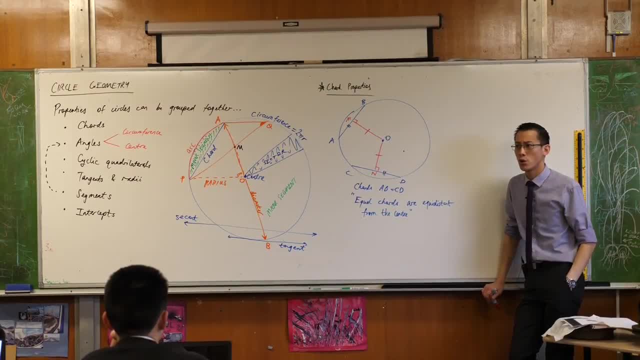 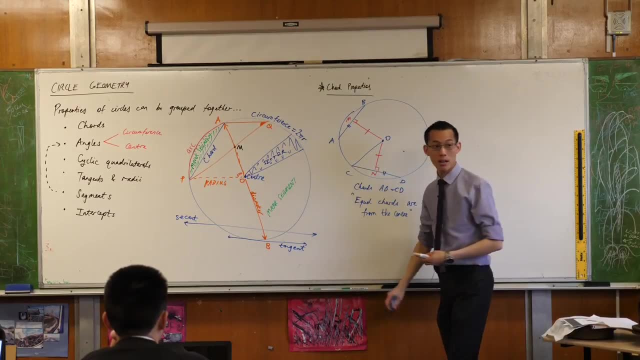 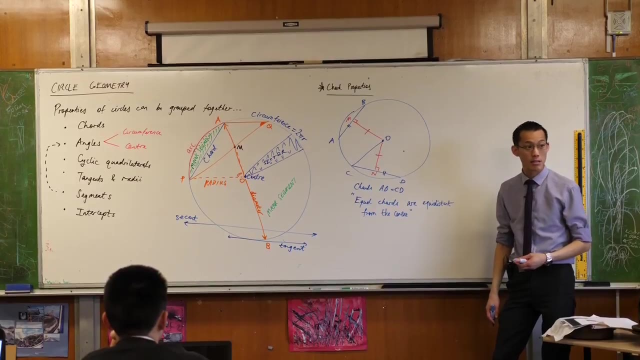 Tell me You've got words, you've got labels. Tell me what I need to join up: C and C and O O, O, O O O, C and C and C and O O O O O, Like that. Is that enough? Do I need to join up anything else? 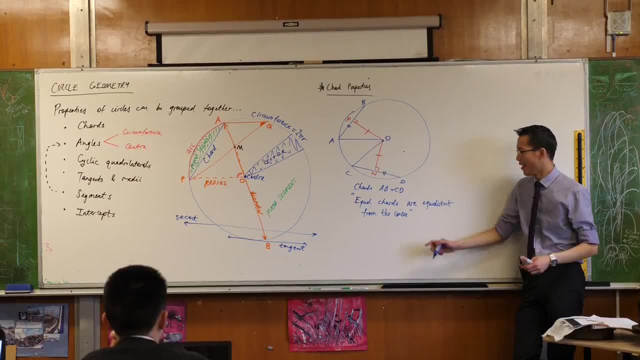 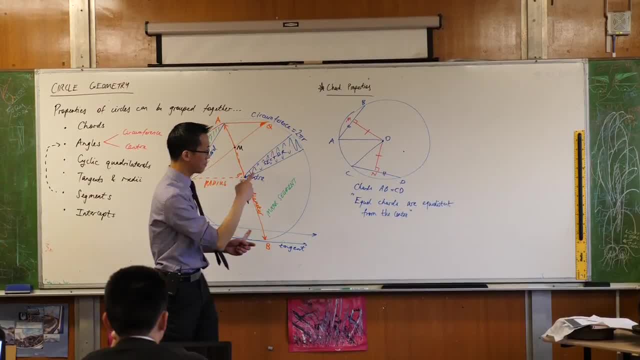 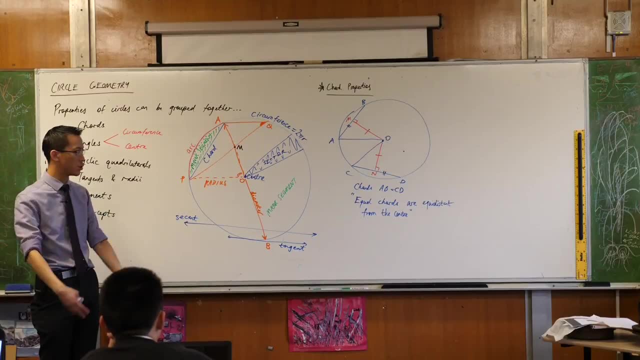 okay, now, as it happens- and this is a property we're going to get to, that perpendicular line does bisect the chord, but i don't know that yet. i'm going to prove that as we go and then, once we proved it, we can use it, but i don't know if that's the case. just yet, if you want to use that, 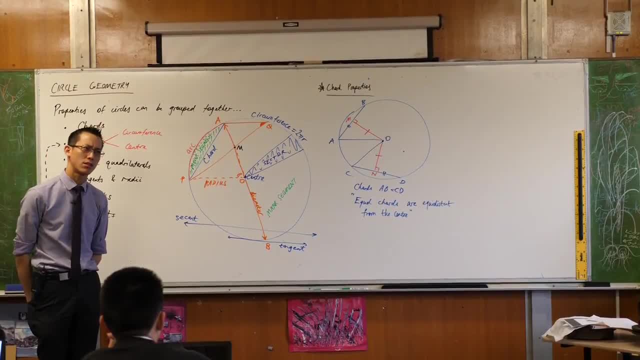 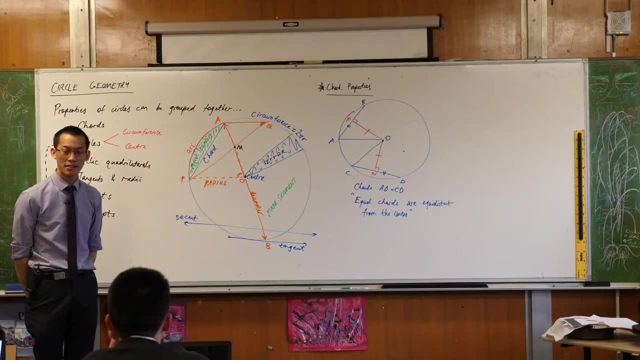 fact. that's okay, but you're going to have to prove it. is there anything else i could do? yeah, what perpendicular formula are you referring to? you guys tell me, yeah, i don't know any formula called the perpendicular formula. um, um, um. okay, so i'm going to pause here. i'm going to pause. this is really interesting, okay. 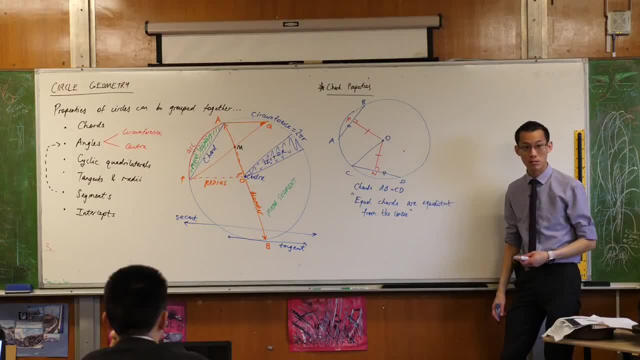 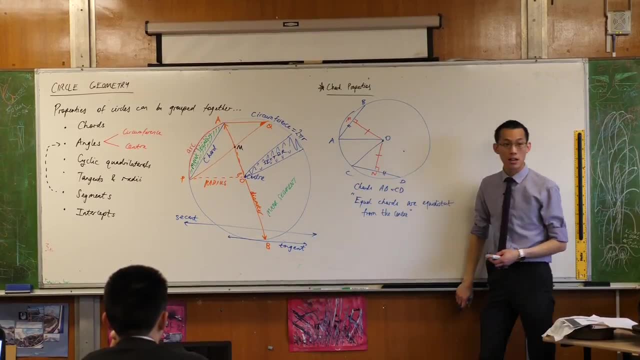 Is that enough? What are you going to do with that? What are you going to do with that? Remember, we don't know anything else about this circle. We're going to have a long list of these eventually, but right now we don't know anything else. 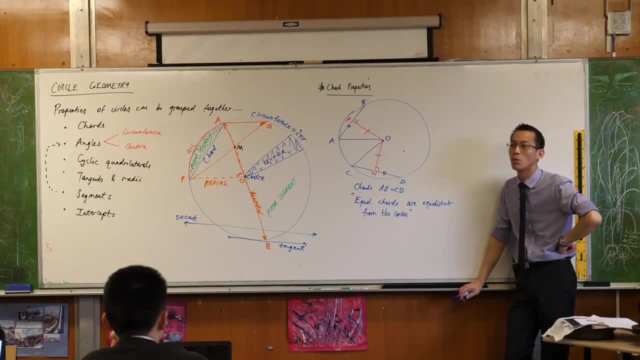 apart from this, We don't know anything else apart from the fact that it's a circle. What else do you want me to do? The quarter equal in the parallel line bisects the right circle. Whoa, whoa, whoa, whoa. 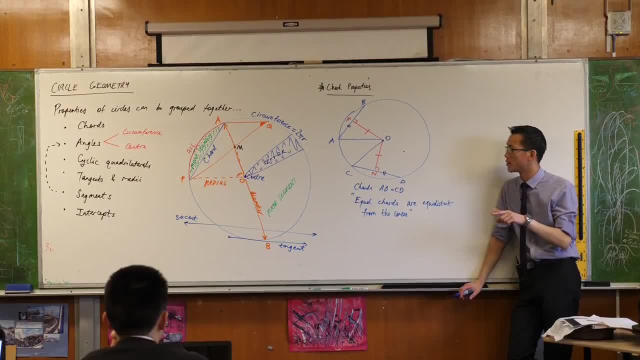 What parallel lines, The right perpendicular line? So you're suggesting this perpendicular line bisects this chord. Is that what you're saying? Okay, Now, as it happens- and this is a property- we're going to get to that perpendicular. line does bisect the chord, but I don't know that yet. I'm going to prove that as we go and then, once we've proved it, we can use it, But I don't know if that's the case just yet. 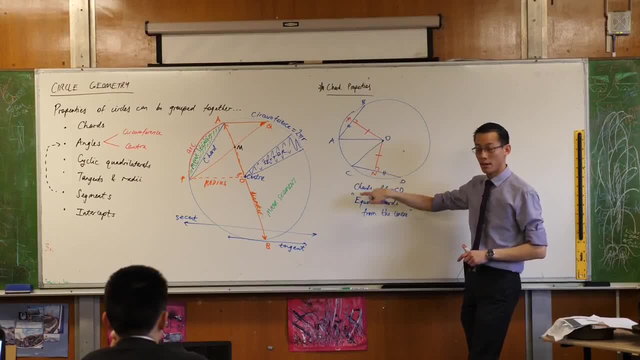 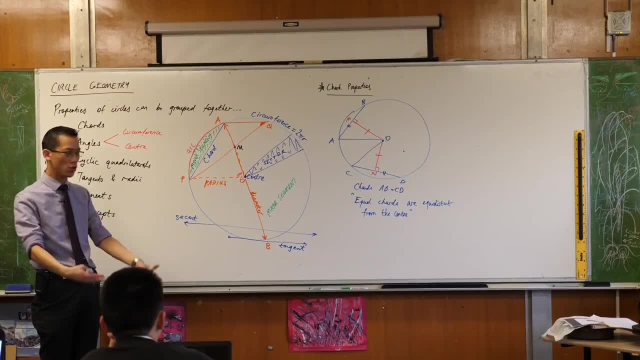 Is there anything else I could do? Yeah, Russell. Well, I don't know if this is right, but if you use perpendicular formula, What perpendicular formula are you referring to? Is there any other one? Well, I don't know if this is right, but if you use perpendicular formula, 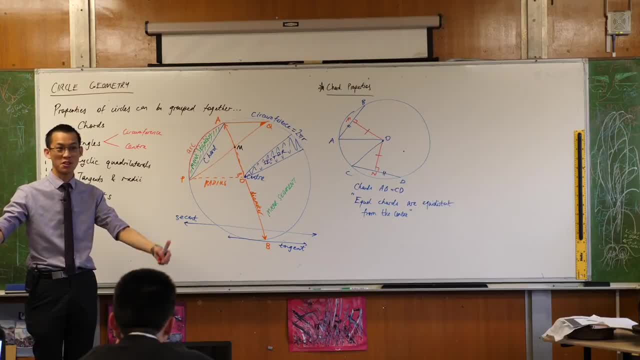 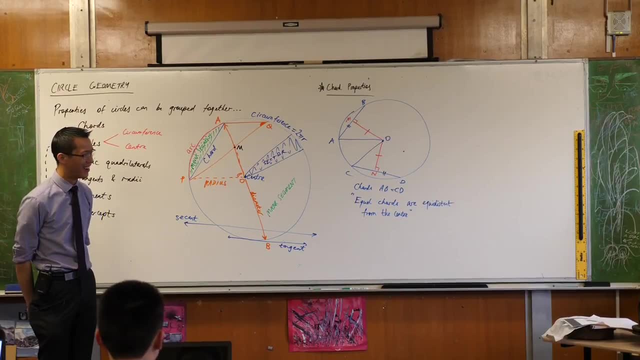 Well, I don't know if this is right, but if you use perpendicular formula, You guys tell me I don't know any formula called the perpendicular formula. Okay, so I'm going to pause here. I'm going to pause. This is really interesting, okay. 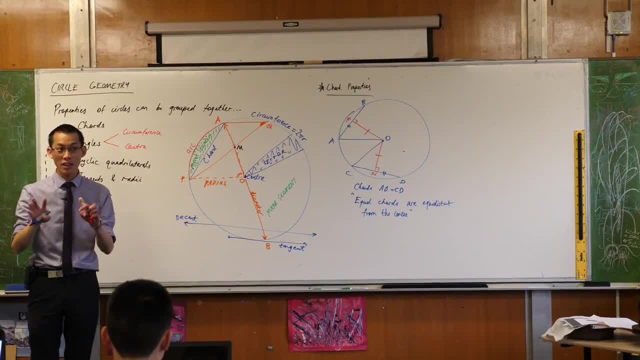 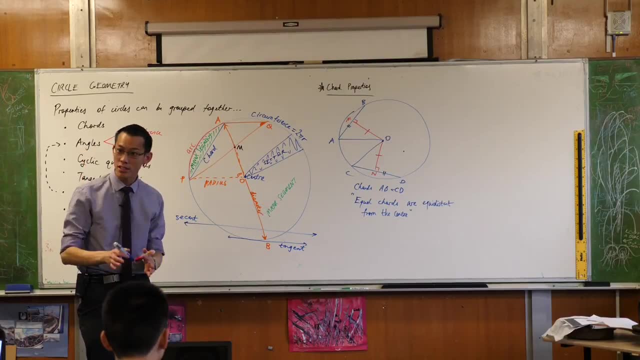 Our diagram is not finished. Well, I'm suggesting it's not finished. I'm going to give you two or three minutes. There's a few different ways to have a go at this. I want you to think about all of the plane geometry knowledge. 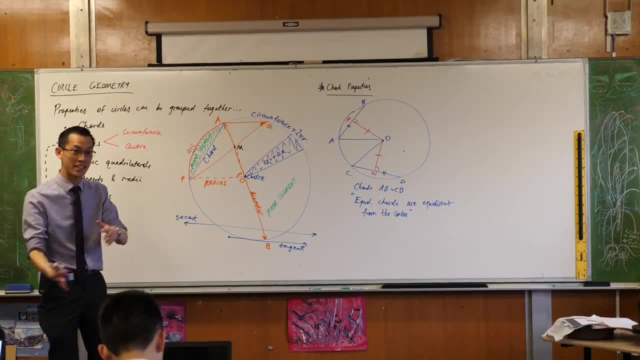 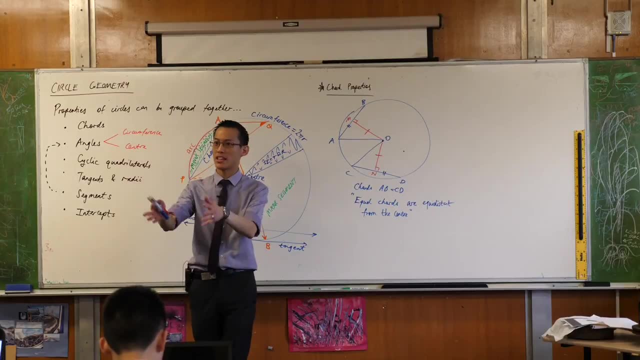 that you developed over the last week and a half or so. That's the reason why we led into that: to get to circle geometry. How would you prove that this is the case, Because it certainly looks like it. Why don't you take some time? 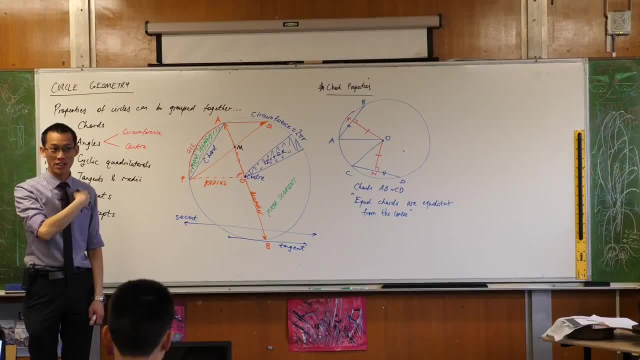 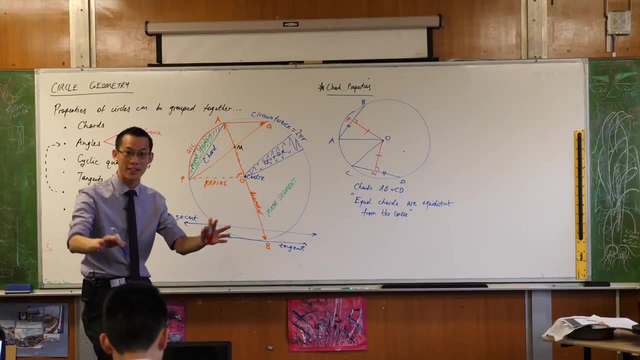 our diagram is not finished. well, i'm suggesting it's not finished. i'm going to give you two or three minutes. there's a few different ways to have a go at this. i want you to think about all of the plane geometry knowledge that you developed over the last week and a half or so. that's the. 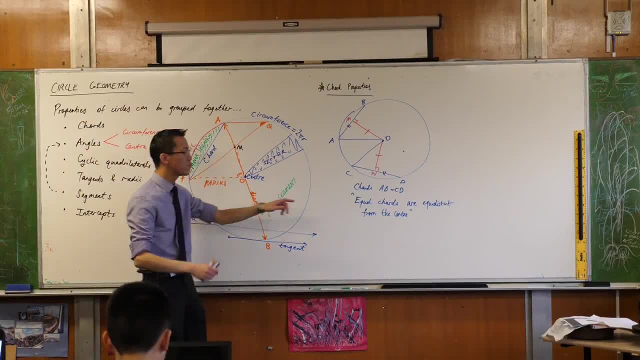 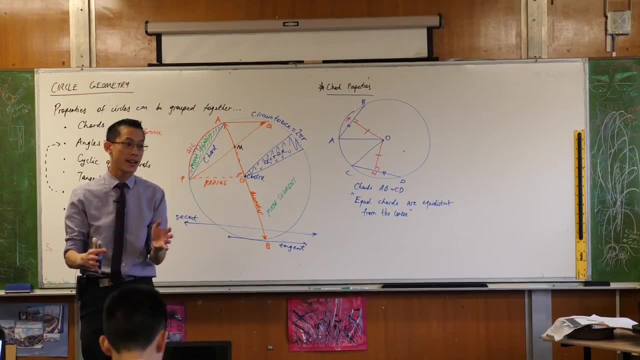 reason why we led into that, to get to circle geometry. how would you prove that this is the case, because it certainly looks like it. why don't you take some time? i'll give you a head start. if you've got an idea, write it down, set it out as a proof, like you normally would. 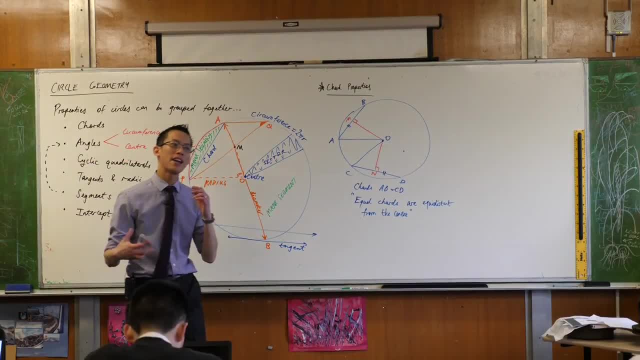 see how far you can get off you go. so, admittedly, part of what's tricky here is we're right at the beginning of this topic, so i'm trying to assume as little as possible. so some things which, in coming days, you will just treat as a given- i'm not treating them as givens yet- for instance the 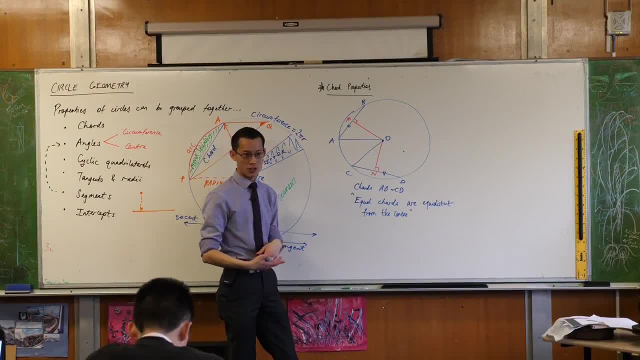 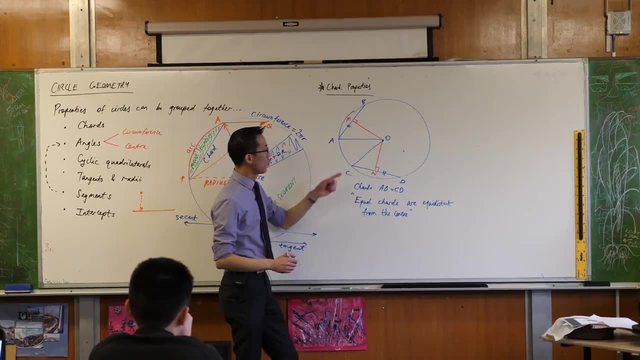 fact that n is in fact in the middle of cd. it's right at the bit it's. it bisects that chord. but we we're going to prove that we're not quite there just yet. so here's what i'm going to do. we constructed o a and o c, these two radii. what i'm going to add to that is that we're going to 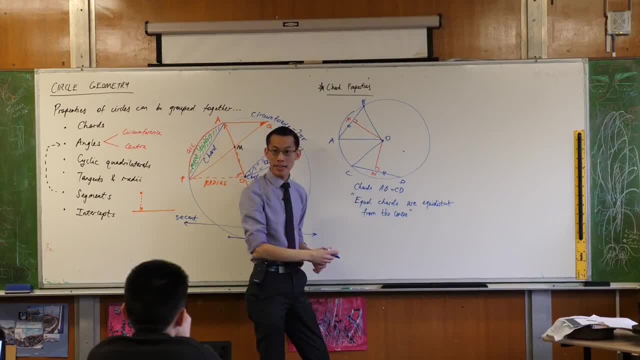 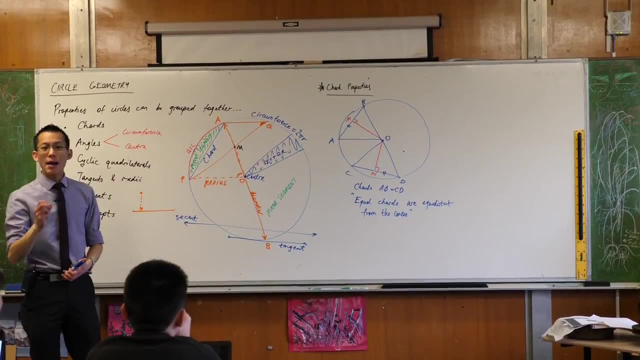 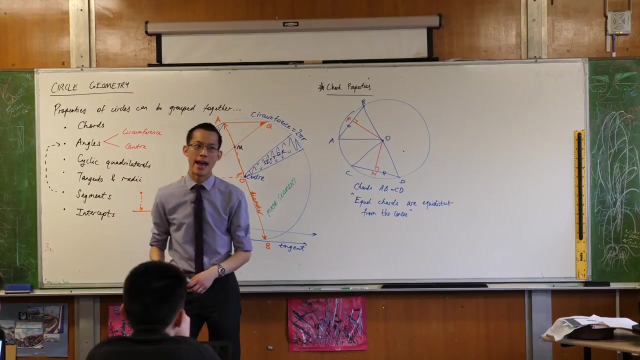 add on to there are ob, that radius and also od. you don't have to do it this way, but it just seems like a pretty straightforward way to go. i'm trying to prove something about distances, right distances. so therefore, when i think about the knowledge that i have that allows me to prove distances, 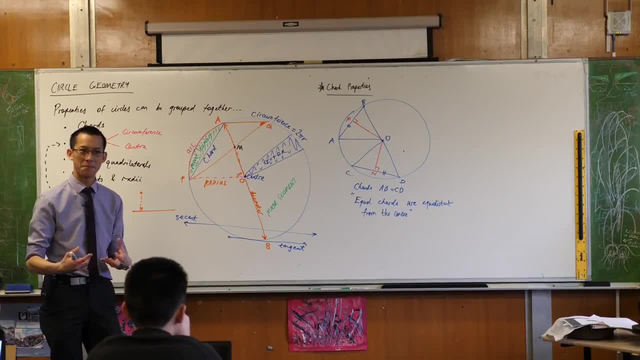 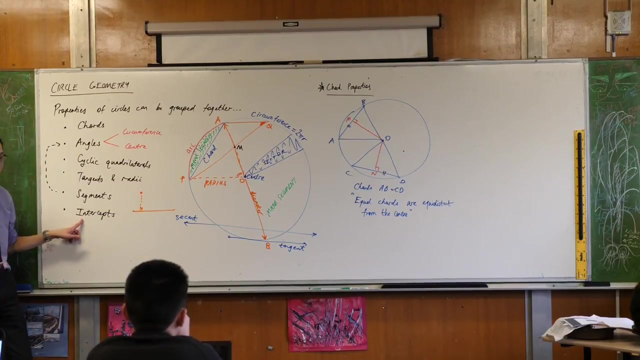 are the same. i need to prove: entire shapes are the same. entire shapes are the same. that's congruence, isn't it? can you see why, for example, similarity is no good for proving something like this? we'll come to similarity. most of the properties about intercepts, for instance, are about similarity, but here, if you want to prove that distances are the 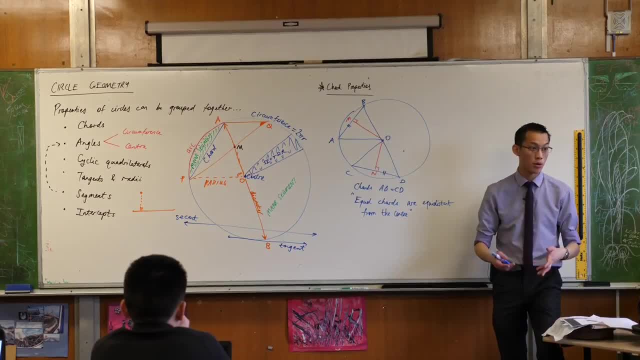 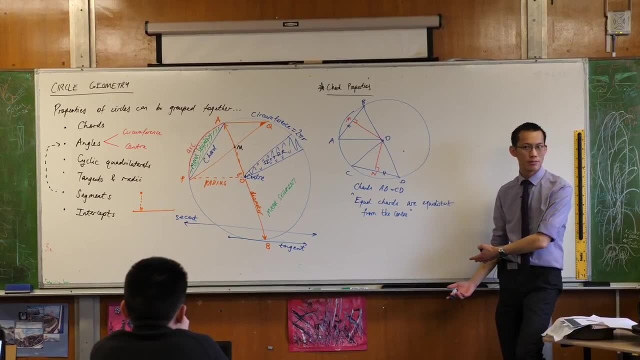 same distances in similar triangles are not the same. they're in proportion. so that's not what i'm after. okay, so what i've done is i've constructed all of these radii and now i've got a pair of triangles. they look pretty congruent, right? can i prove that they're congruent? i can't, can't i? 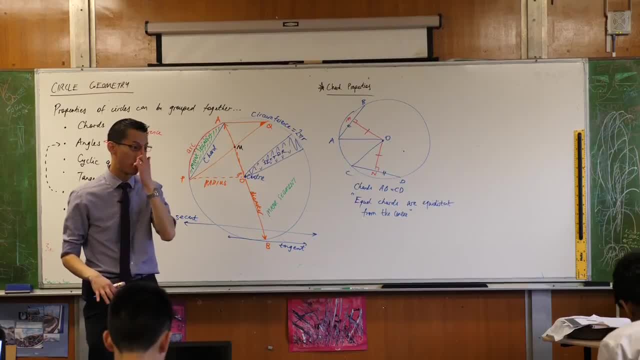 I'll give you a head start. If you've got an idea, write it down, Set it out as a proof, like you normally would See how far you can get Off you go. So, admittedly, part of what's tricky here is we're right at the beginning of this topic. 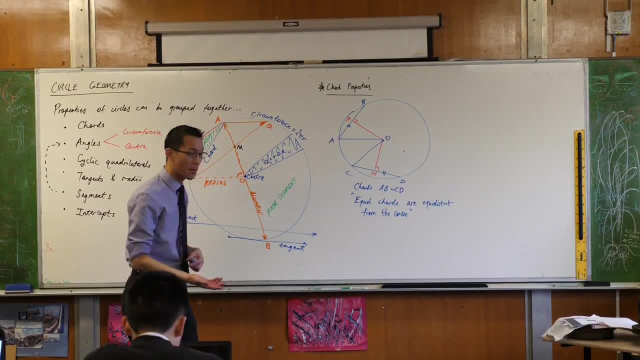 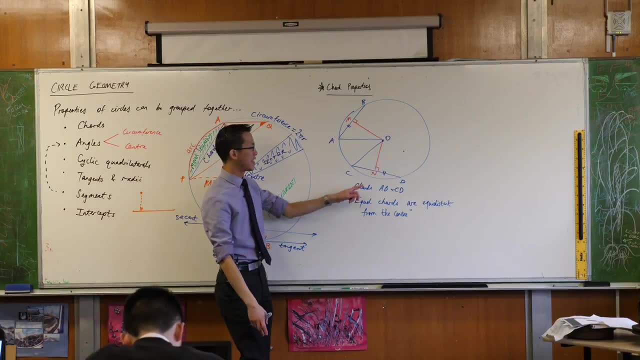 so I'm trying to assume as little as possible. So some things which in coming days you will just treat as a given, I'm not treating them as givens yet. For instance the fact that n is in fact in the middle of cd. 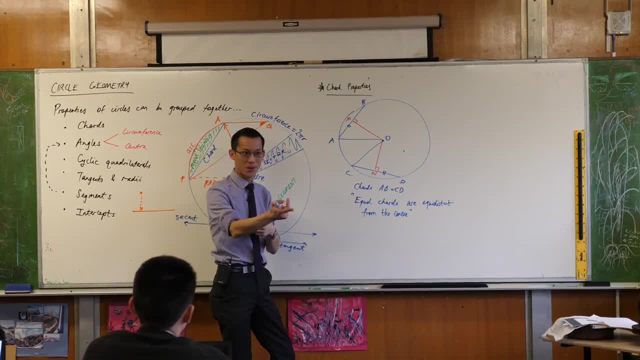 It's right at the middle. It bisects. It bisects that chord, But we're going to prove that We're not quite there just yet. So here's what I'm going to do. We constructed oa and oc, these two radii. 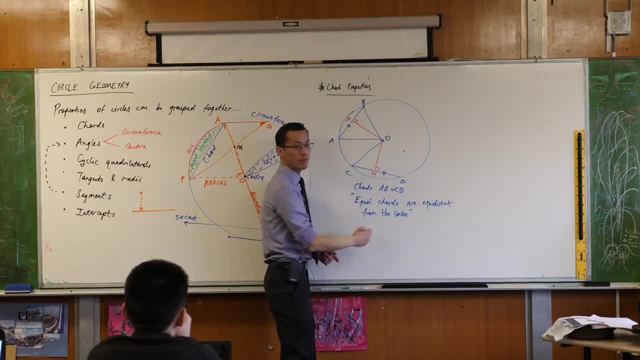 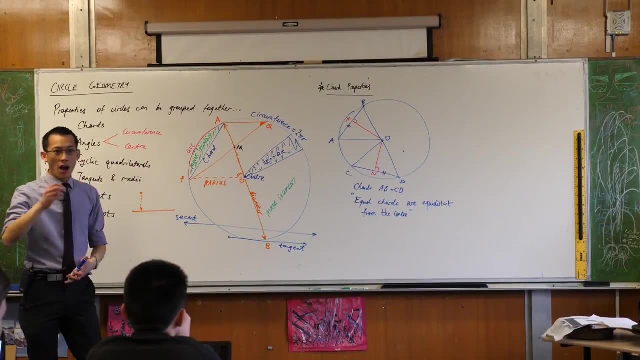 What I'm going to add on to. there are ob, that radius, and also od. You don't have to do it this way, but it just seems like a pretty straightforward way to go. I'm trying to prove something about distances, right. 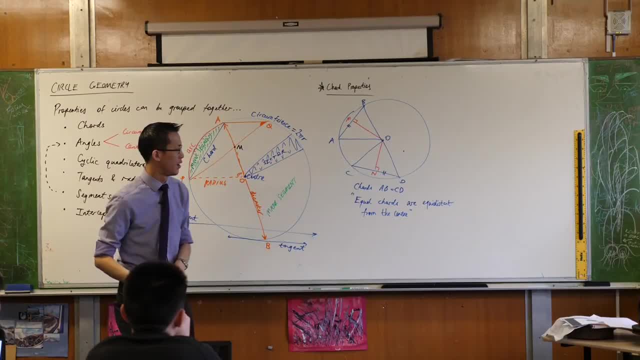 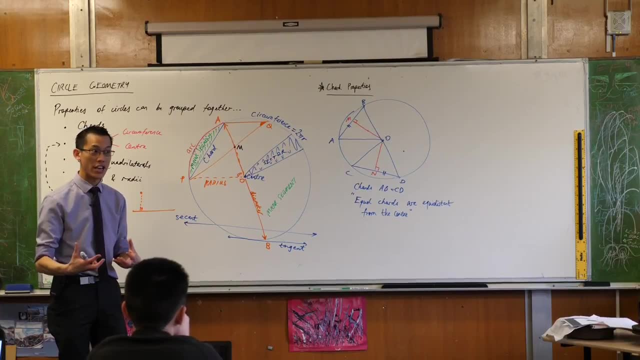 Distances. So therefore, when I think about the knowledge that I have that allows me to prove distances are the same, I need to prove: entire shapes are the same. Entire shapes are the same. That's congruence, isn't it? 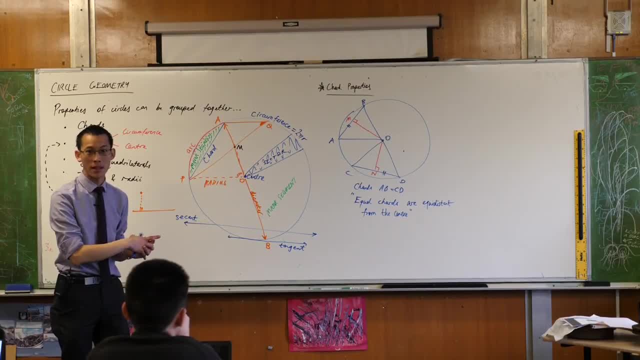 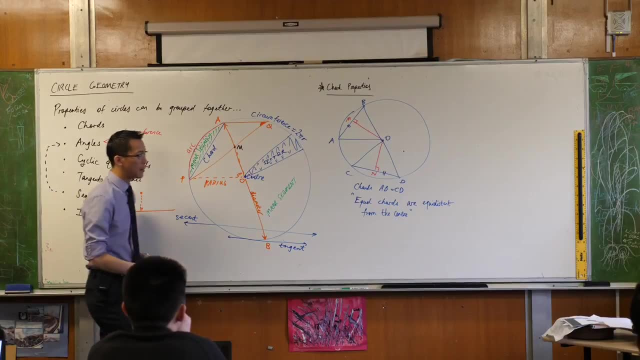 Can you see why, for example, similarity is no good for proving something like this? We'll come to similarity. Most of the properties about intercepts, for instance, are about similarity, But here, if you want to prove that distances are the same, 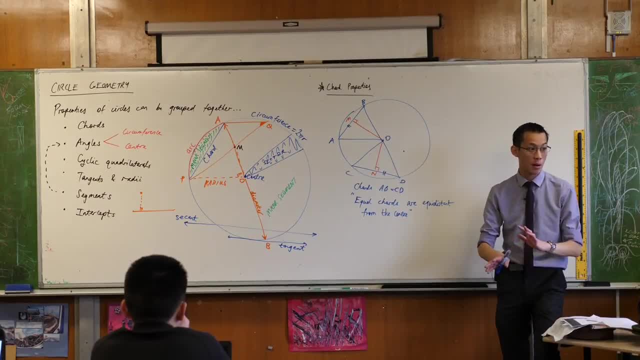 distances in similar triangles are not the same. They're in proportion. So that's not what I'm after. So what I've done is I've constructed all of these radii and now I've got a pair of triangles. They look pretty congruent, right. 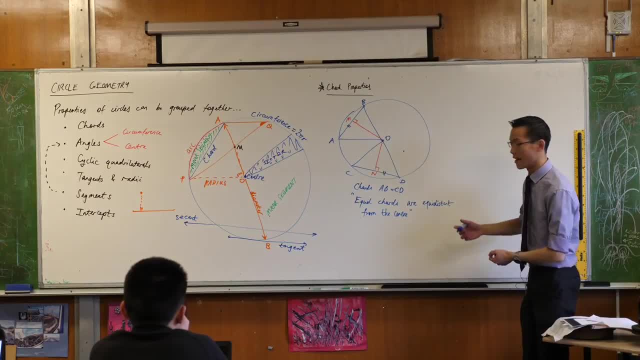 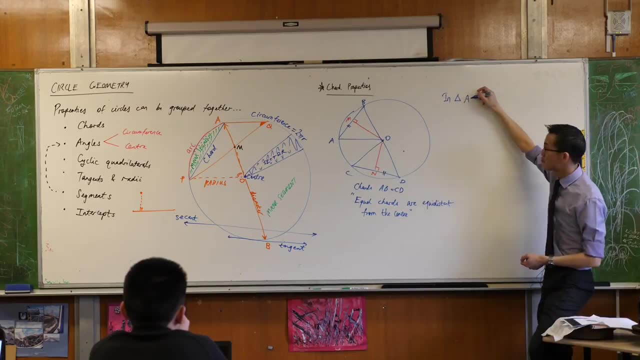 Can I prove that they're congruent? I can, can't I? What would you like to call these triangles? Let's call the top one A, B, O And, if we're doing it in the same order, down the bottom. 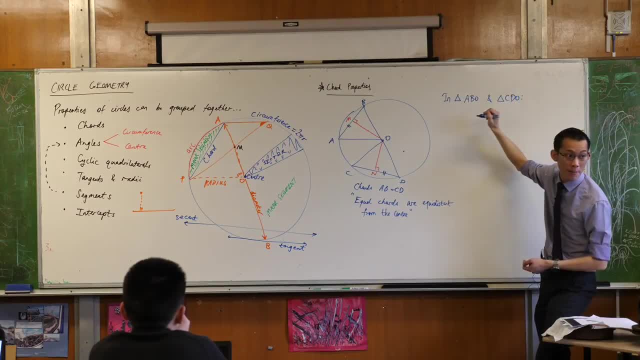 C, D, O, I'd guess right, Because you can see these guys are the chord, so they correspond to this chord. All fine, In these two triangles, what have I got? Well, A, B does equal C, D. 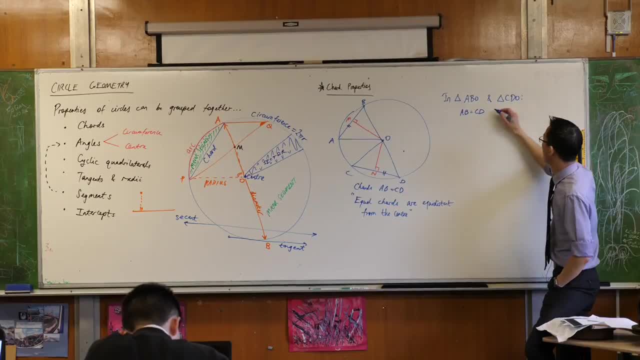 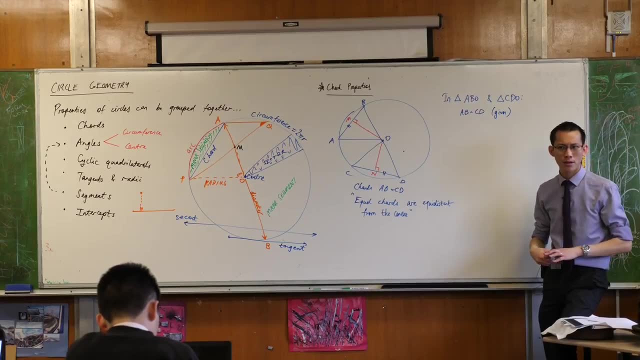 That's the way that we actually constructed this. That's where this diagram comes from, So I can say that's given. I'm going for congruence. What other kinds of features do I have that I know are the same. Yeah, Celine. 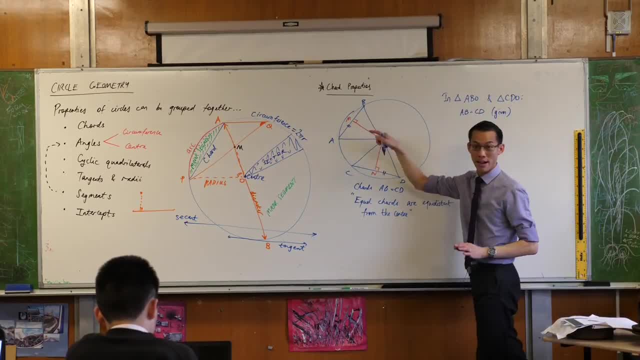 Good. So most of you have spotted, I do have all of these radii that are equal to each other, So I'm going to go for A O being equal to. I'm looking at the letters, because I did the work up here. 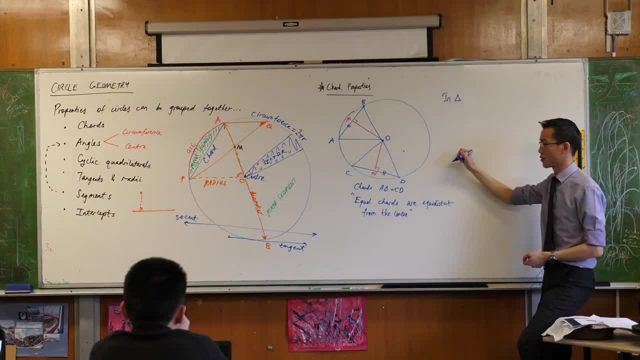 what would you like to call these triangles? let's call the top one a, a, b, o, and if we're doing it in the same order, down the bottom, c, d, o, i'd guess. right, because you've got. you can see, these guys are the chord, so they correspond to this chord. all fine in these. 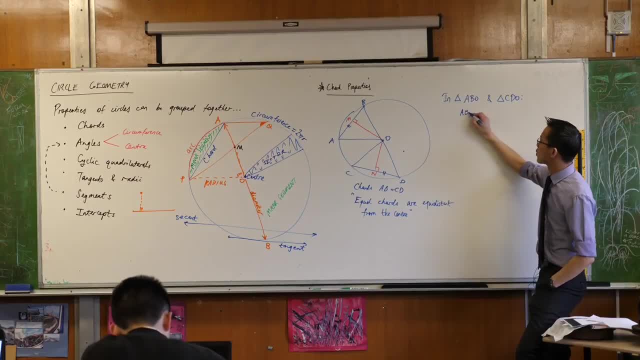 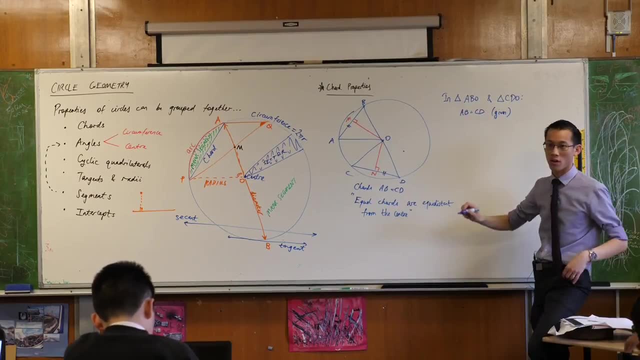 two triangles. what have i got? well, a, b does equal c d. that's the way that we actually constructed this. that's where this diagram comes from. okay, so i can say: a b does equal c d. that's the way that we. that's given. all right, i'm going for congruence. what other kinds of features do i have that i? 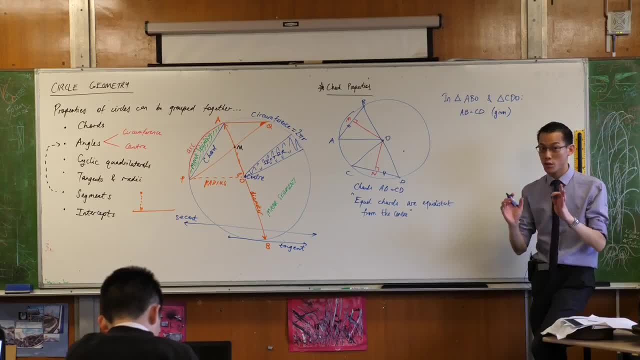 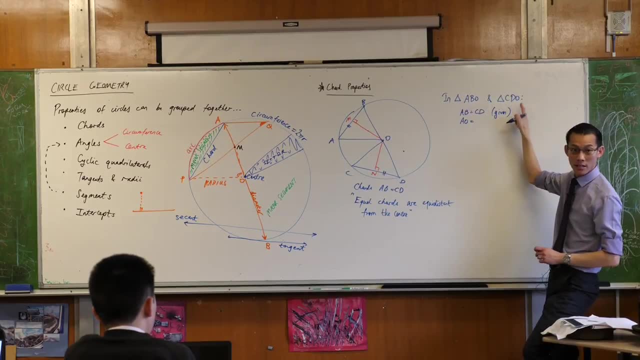 know are the same. yeah, celine, good, so most of you have spotted i do have all of these radii that are equal to each other, so i'm going to go for a o being equal to. i'm looking at the letters, because i did the work up here to make sure the letters are in the right order. i can just quote the: 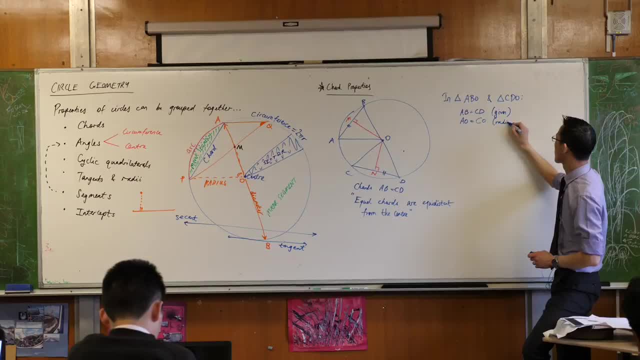 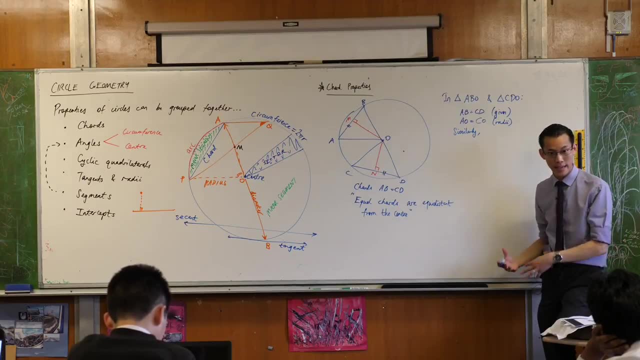 letters in the same order. down here they're radii. similarly, and we use this word in different ways. right, so that what's that? the same is equal to i, and i can justuden out, when you write r and d, what's my particular congress reason is s s, s. so there are two. 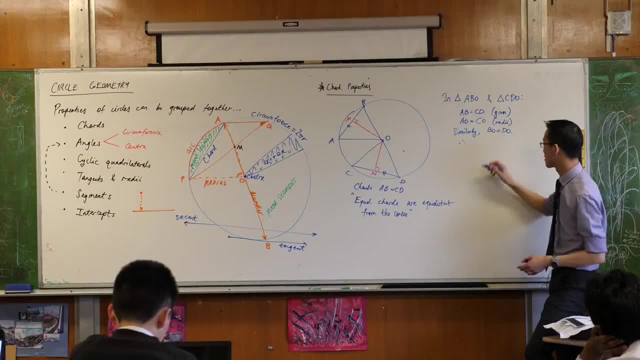 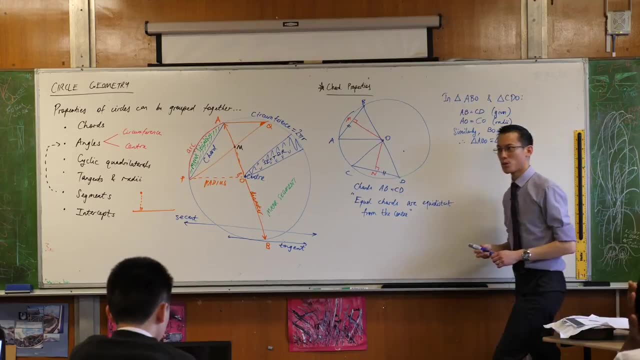 This is at done. the second part you said's and this is at two, and we've still got these two triangles. and the final reason is sc, the second part to the relations 기분. Look at this over here: these two triangles are the same place, so i got these two triangles. 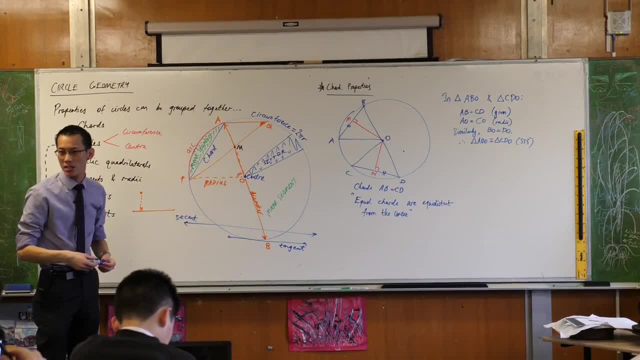 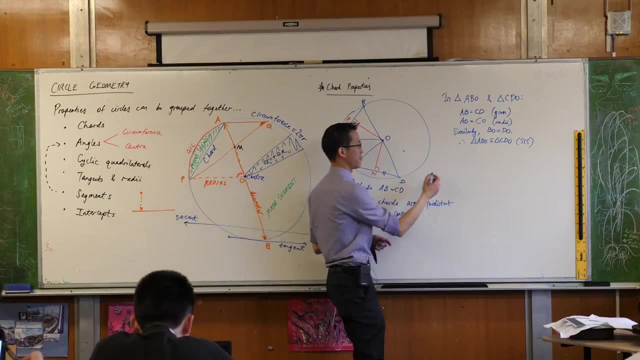 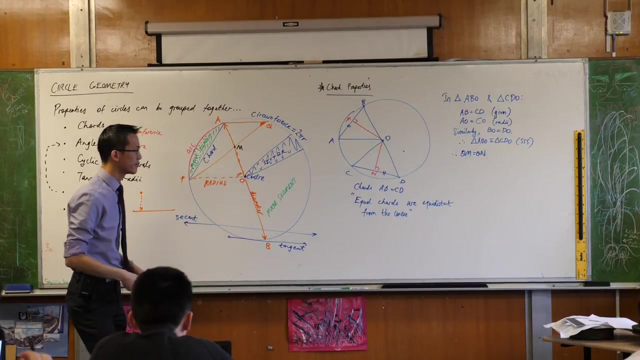 at a different time. it's correct around, rotated a little bit, as it turns out. so how do I get to the thing that I want? because it's pretty much the next line. what's the reason? I think I heard it so you can't say anything about. 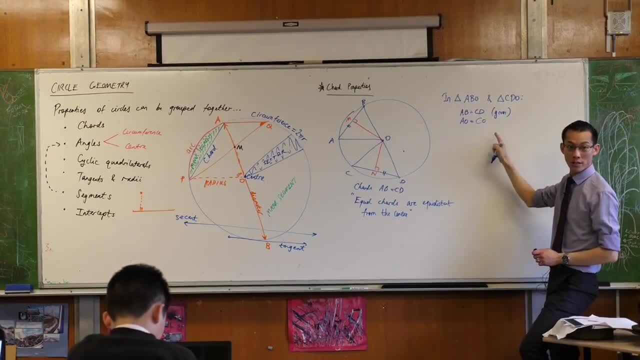 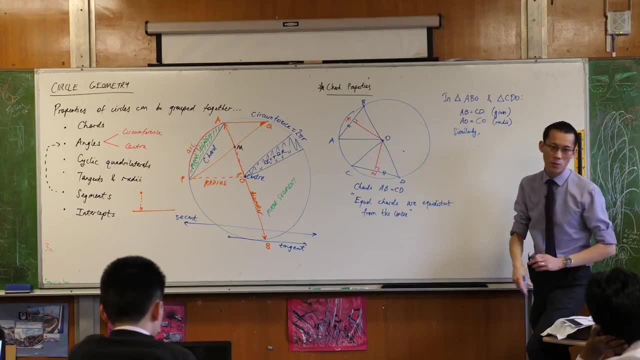 to make sure the letters are in the right order. I can just quote the letters in the same order. down here They're radii. Similarly- and we use this word any time- the reasoning for what I'm about to say is identical to the reasoning that I just said. 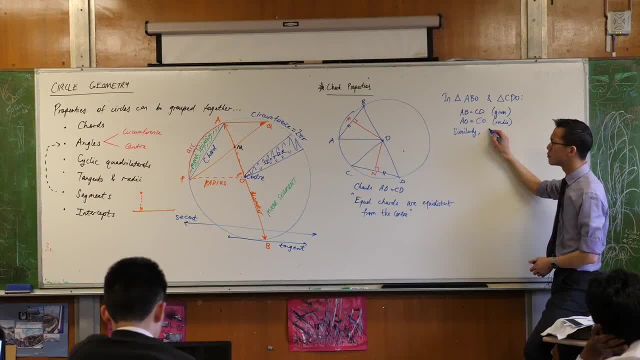 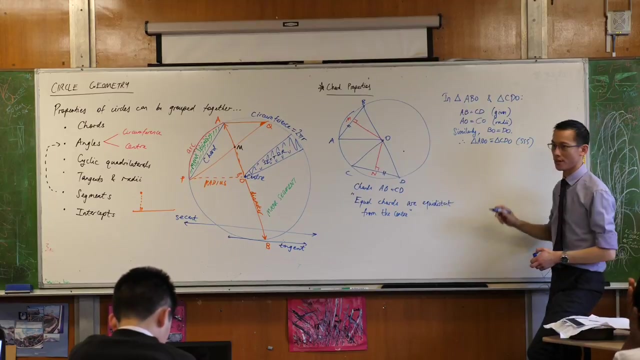 Similarly, what's the other radii that I have? I've got B, O and D? O, right. So therefore, what's my particular congruence reason? S, S, S. Okay, So now I know that these two triangles are exactly identical. 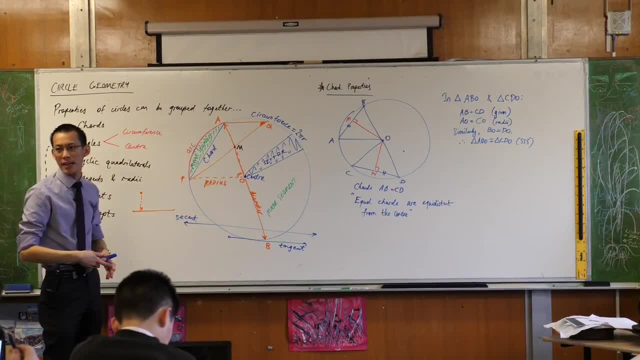 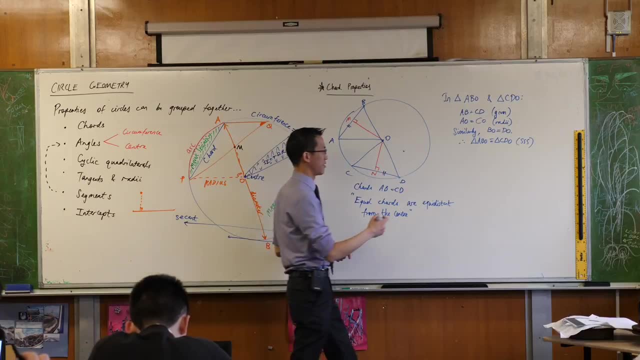 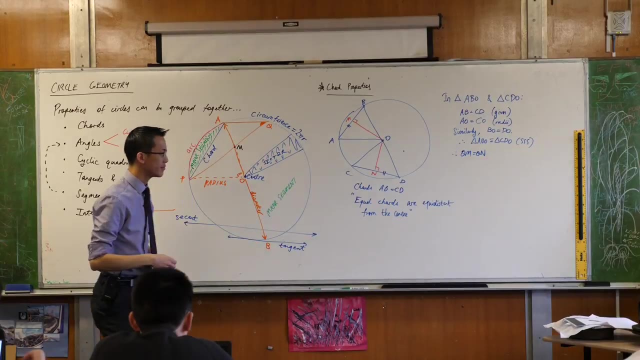 in every way. They've just been shuffled around, rotated a little bit, as it turns out. So how do I get to the thing that I want? Because it's pretty much the next line. What's the reason? I think I heard it. 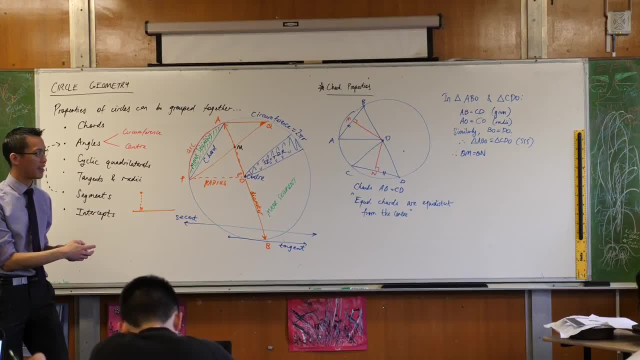 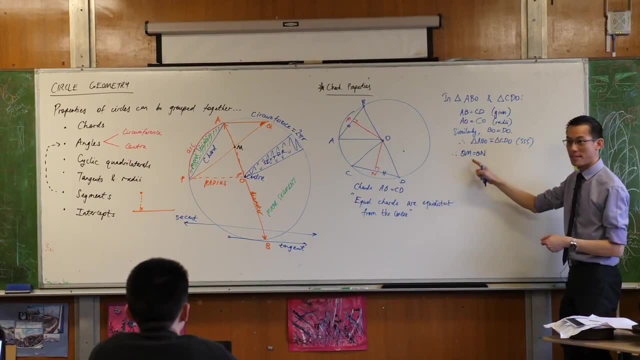 So you can't say anything about corresponding sides, because I, O M and O N are not sides in this triangle. okay, However, I can say if O M is equal to O N or the reason why O M is equal to O N. 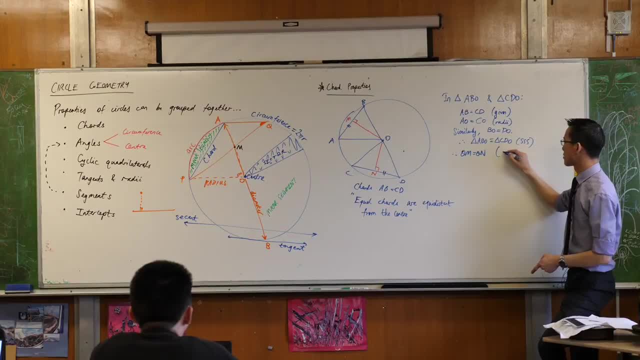 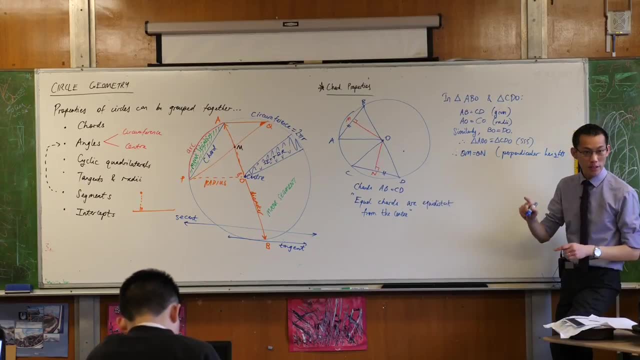 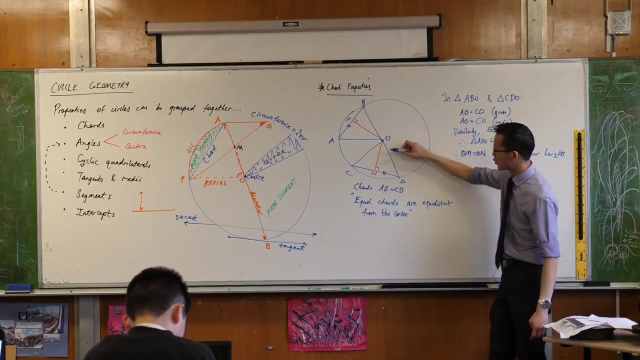 is because both of them are perpendicular heights And, importantly, they're corresponding perpendicular heights because we know there's actually different ways that you can refer to the height of a triangle. I could have drawn it this way and made it perpendicular as well. 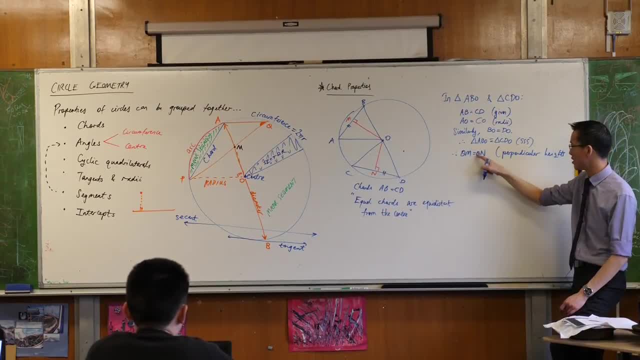 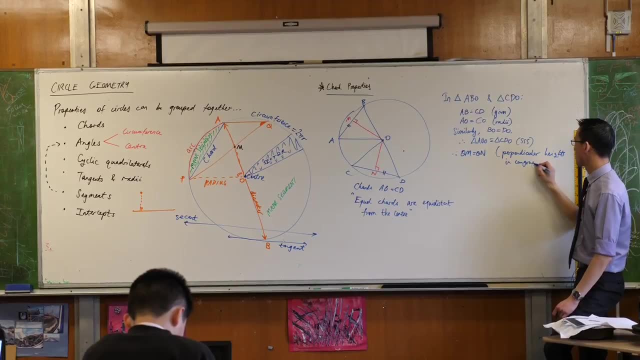 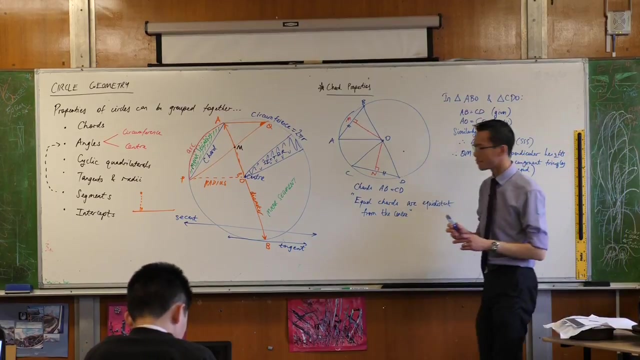 It would be just as valid. But they're the same orientation, right? You can see everything matches up. So O, M and O N are perpendicular heights in congruent triangles. Okay, That's all you need to say. Okay. 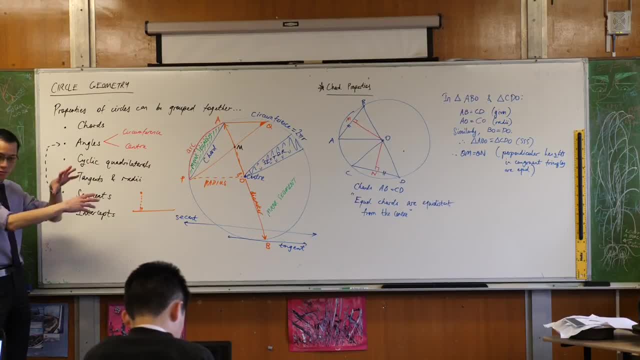 Now I want you- I'm going to stop talking at you, because I just wanted to show you what I was talking about here- I want you to now file this away as true. I can rest on this now. It's proven. 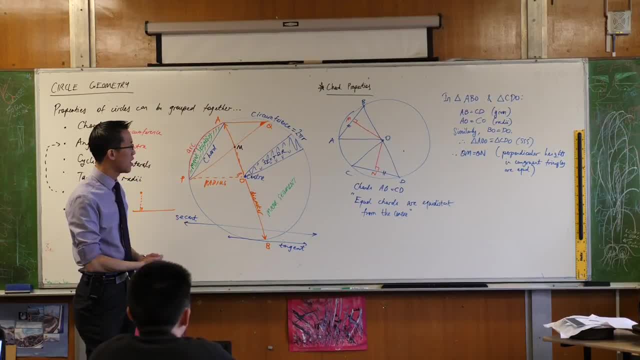 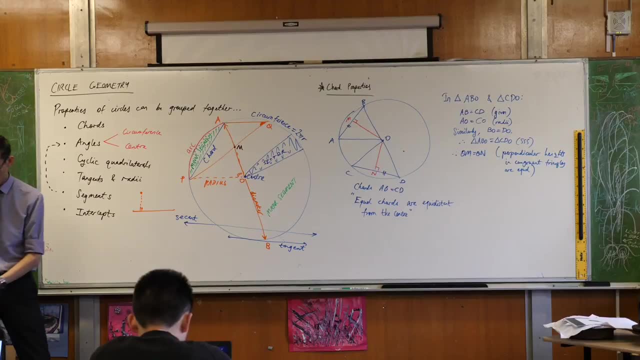 So I can use this as a further tool in my toolbox. You've got a few other chord properties. They start from page 347, or 347 on the textbook, I don't know what it is on the PDF. You can see. we proved the first one. 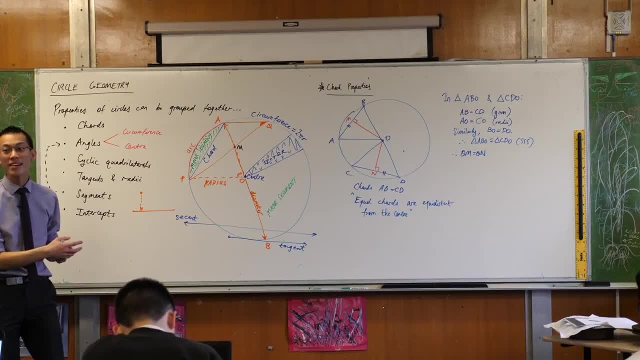 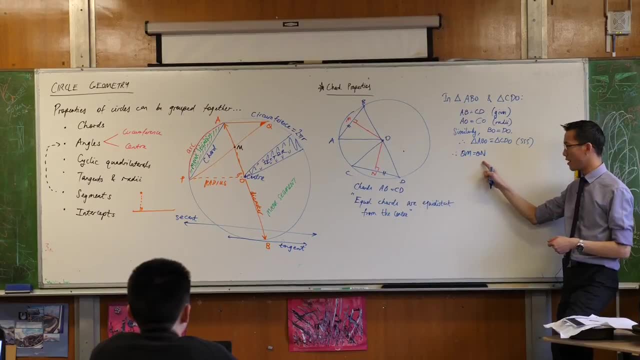 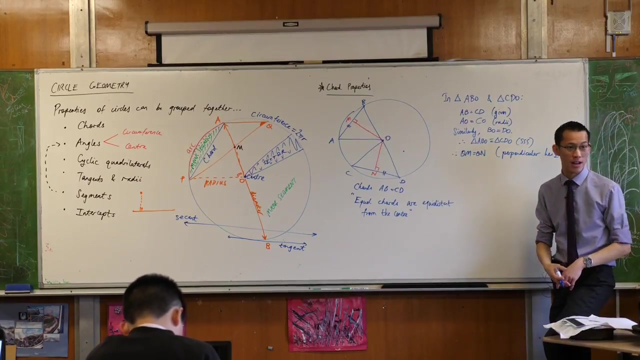 corresponding sides, because I, om and om are not sides in this triangle. okay, however, I can say: if om is equal to om, or the reason why om is equal to om, is because both of them are perpendicular Heights and, importantly, they're corresponding perpendicular Heights because we know there's actually 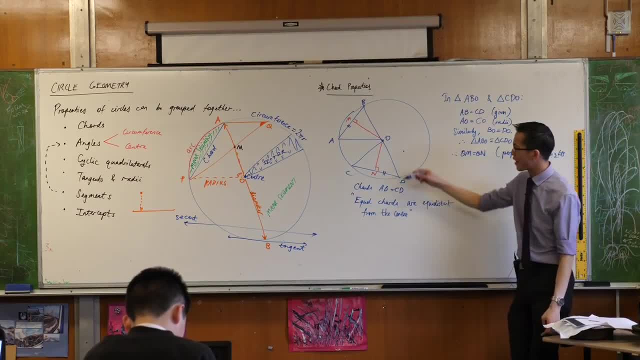 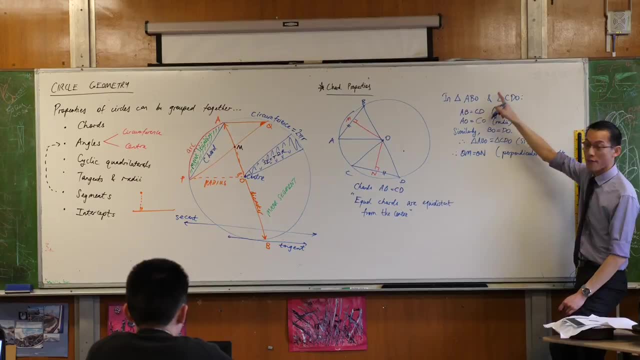 different ways that you can refer to the height of a triangle. I could have drawn it this way and made it perpendicular as well. would be just as valid, but they're the same orientation, right? you can see? everything matches up. so, om and on are perpendicular Heights in congrove. 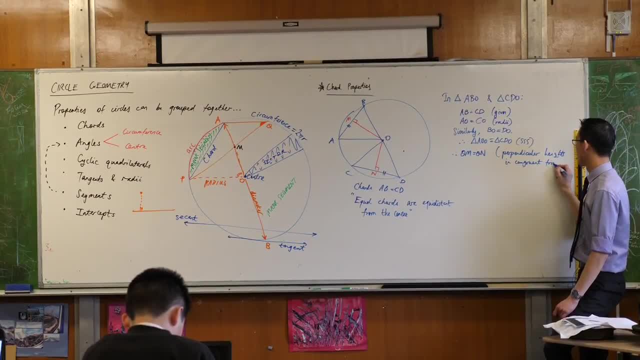 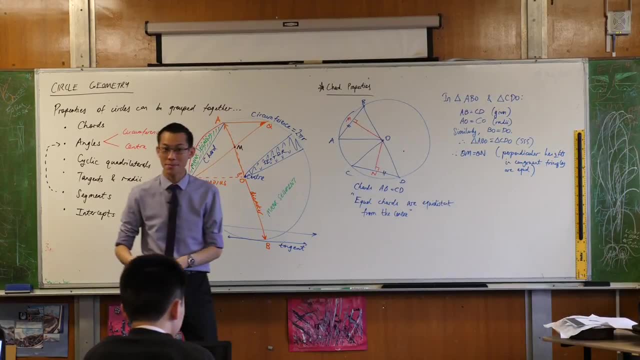 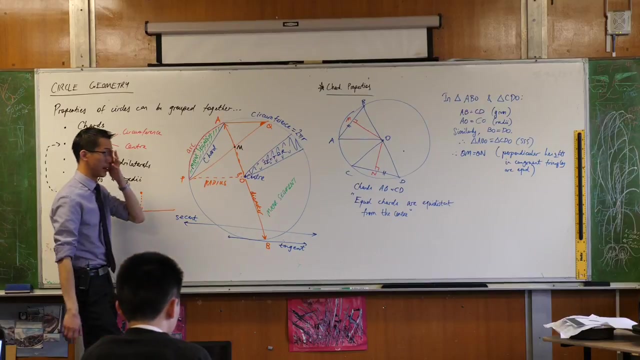 triangles. that's all you need to say. okay, now I want you. I'm gonna stop talking at you, because I just wanted to show you what I was talking about here. I want you to now file this away as true. I can rest on this now. it's proven, so I can use this. 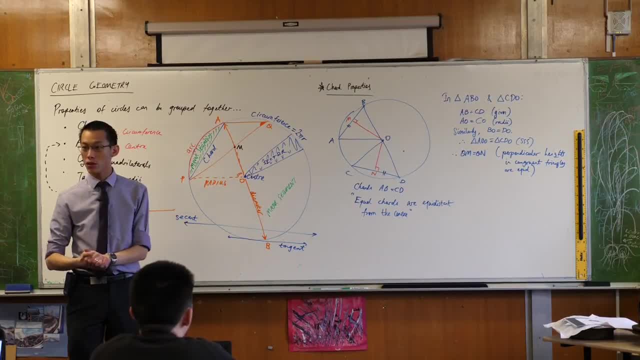 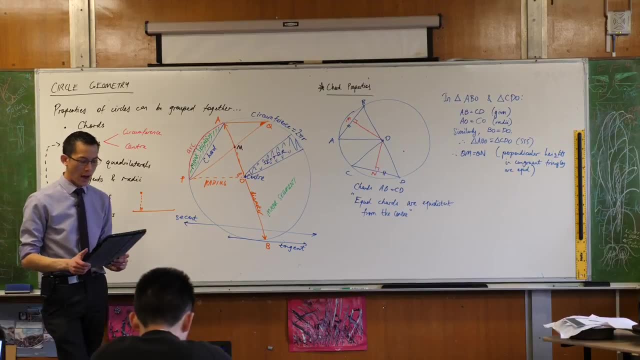 as a further toulouse in my toolbox. you've got a few other chord properties. they start from page 347 or 347 on the textbook, I don't know what it is on the PDF. um, you can see, we proved the the first one. chords and distance from the center, one of the 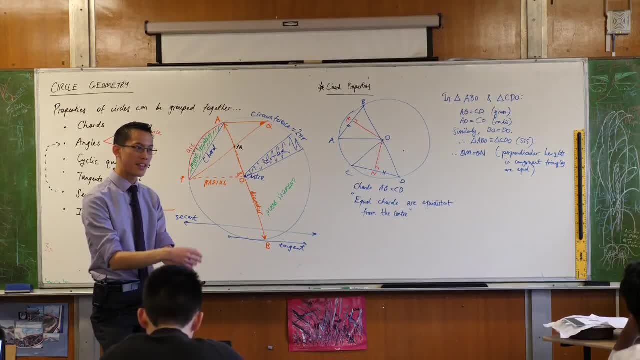 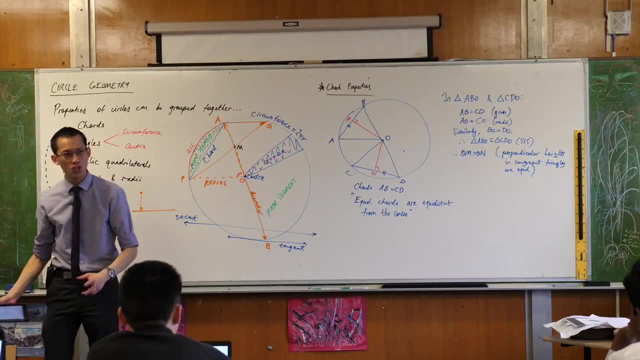 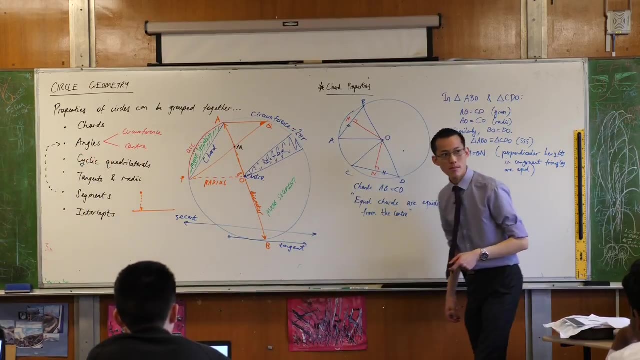 really nice things are. pretty much every circle property. is that the converse is also true. what would the converse of this theorem be? or property? how would you state it in Reverse? yeah, Eric, what do you think? yeah, that's you. you got all of that. you got the order right. you got this, the 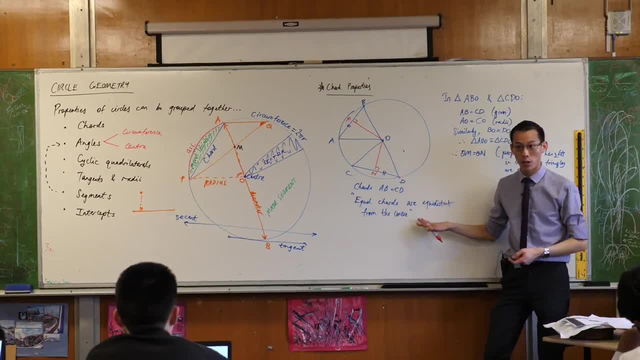 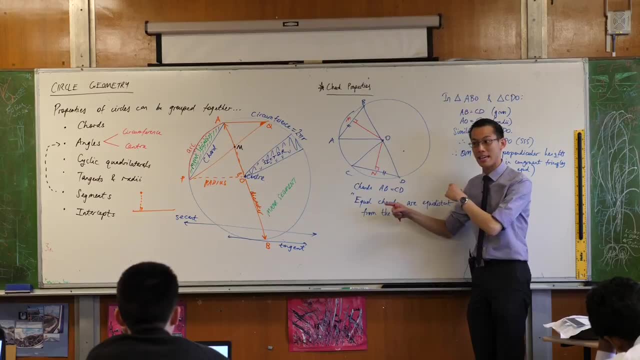 sentence a little bit awkward, but I put you on the spot. the whole idea here was we started with equal chords and then we concluded something about their distance from the center. okay, well, to say the converse is to do that in reverse order. so the way I'd say it- you're what going to put this underneath as well- is if you